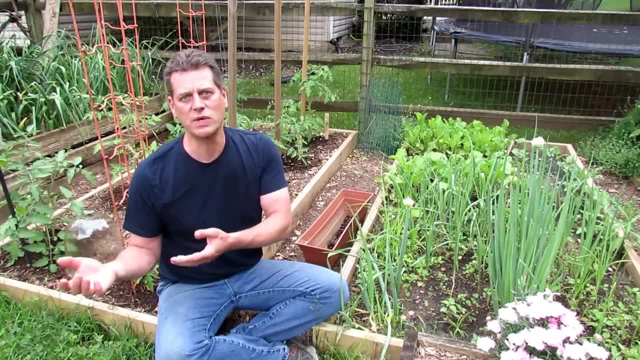 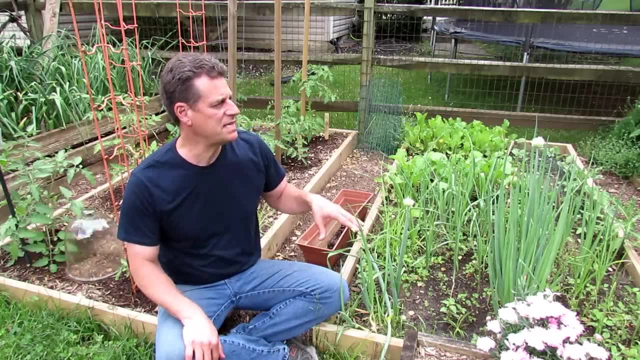 I'm going to take you to Nashville, Tennessee, where I was this weekend, where I dug a garden for my son and got it planted up. Before we get to that, I want to show you a quick tour of the space here, give you an idea of some of the sizes of the different beds I have. 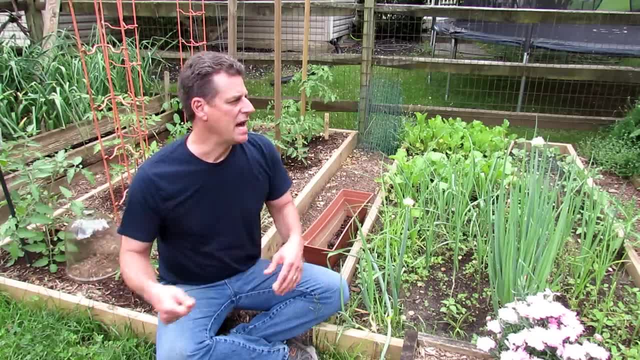 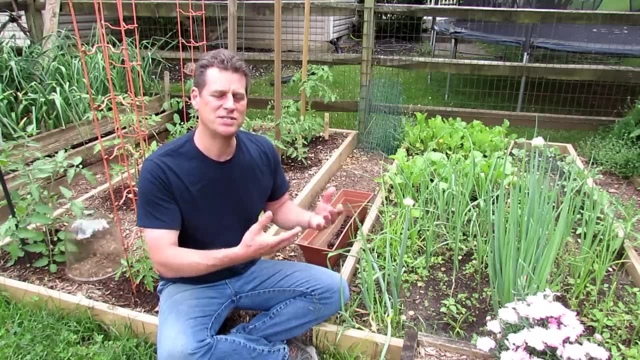 so you can decide what you want to put in your yard. And then I'm going to just show you how to blend any bagged soil you get from stores with your earthbed soil. It's an important principle that once you understand it, it makes perfect sense. 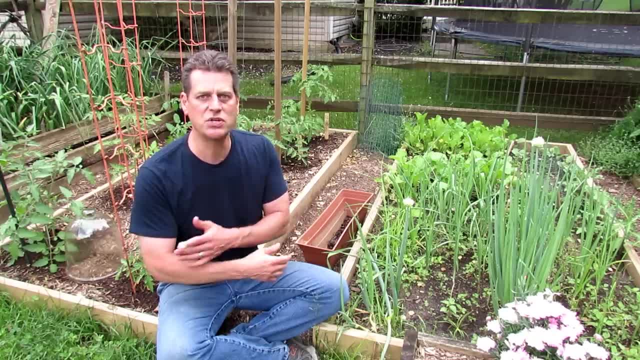 So let's get to the beds, and then we'll get to Nashville and I'll show you all the steps needed to dig your first garden and plant your first garden. So these are raised beds. You don't have to build raised beds. 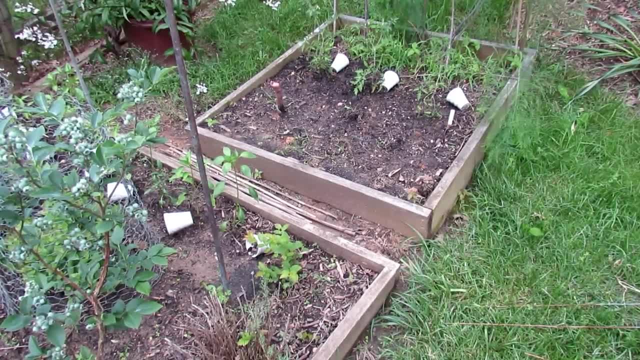 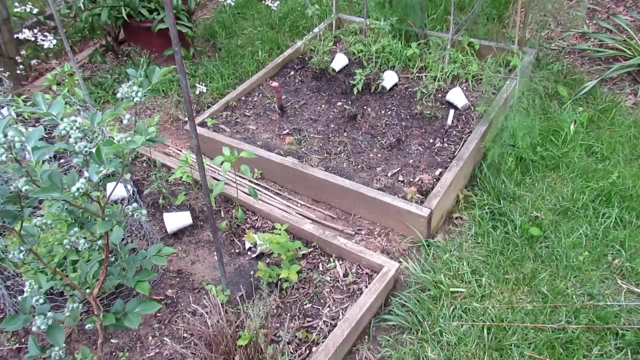 If you want to build a raised bed, you can go to Home Depot or Lowe's and ask them to cut the wood for you, and you just basically put screws in the side. There's plenty of videos on building raised beds, But let's just pretend this is an earthbed, because that's what I want you to start with. is just go right to your ground. That's a 4x4 space right there. You want it to be 4 foot by 4 foot, or you want a 4 foot by 8 foot. By keeping it those dimensions, you can reach into your garden and tend it without walking in the space. 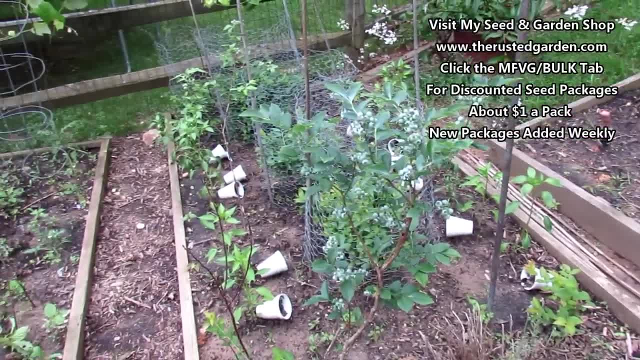 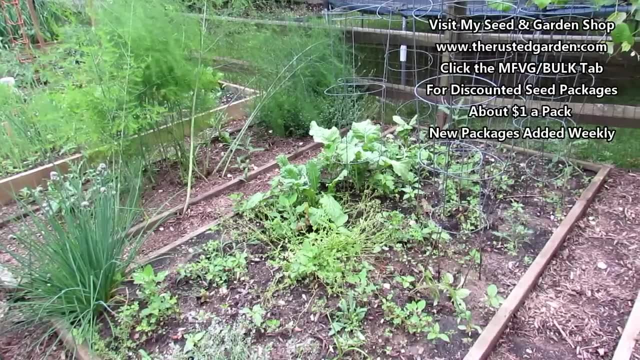 But that's a 4x4.. This is an 8 foot by 4 foot garden And this is the space we're going to fix up. It's also an 8 foot by 4 foot space. Essentially, what you want to do is pick the space. watch the video. 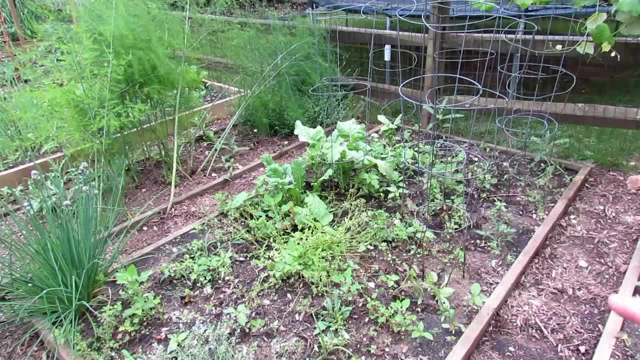 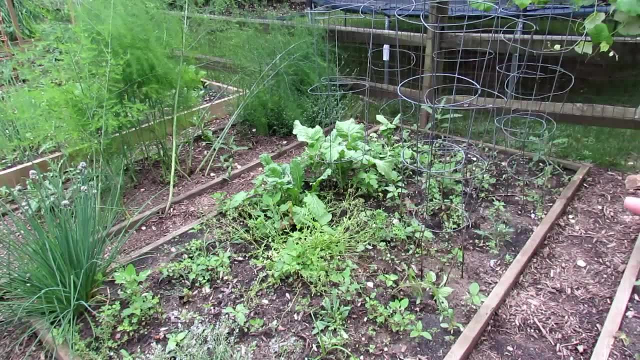 It'll tell you where to pick the best spot for your garden. Remove the greenery. You can either put down cardboard and kill it off over a six week period, You can whack it down with a weed whacker. But remove the greenery and then turn the soil. 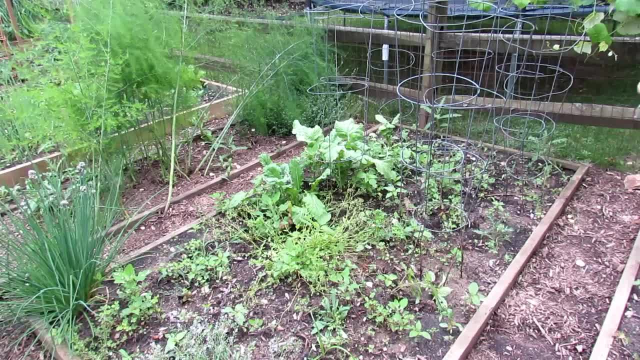 Sounds simple, but when you don't know how to do this, you don't know how to do it, So let me just show you. So we're going to clear this out and start turning the bed, and then we're going to add in the garden bag soil. 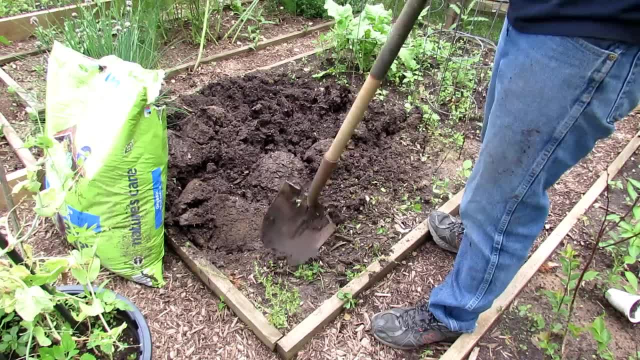 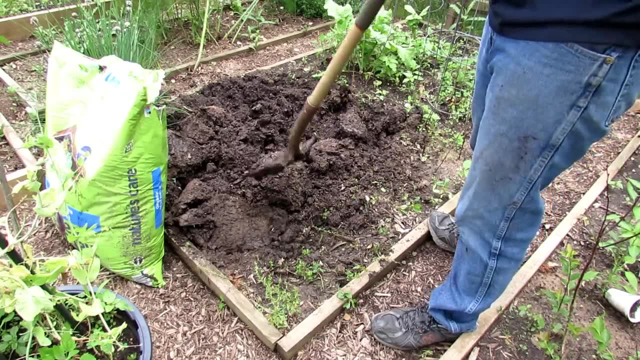 So I'm just turning a 4 foot by 4 foot space. That's plenty of room to get in two tomatoes, two pepper plants and even a couple of herbs. So you're going to clear off the grass. You can, you know, cut it down with a weed whacker. 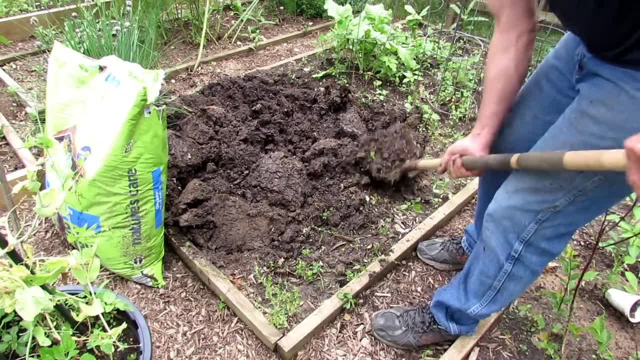 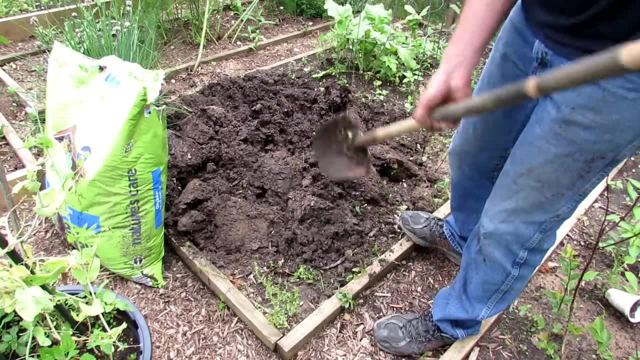 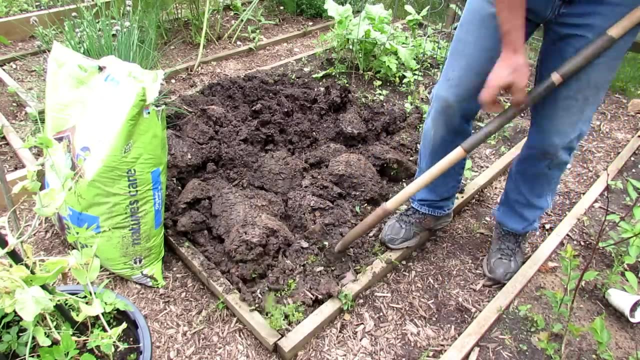 Just turn it over, and once you cut the grass down, turn it over full length of a shovel, Loosen it up. Now, of course, this bed's been prepared, So if you have You know soil that looks like this, you may not have to amend it a whole lot. 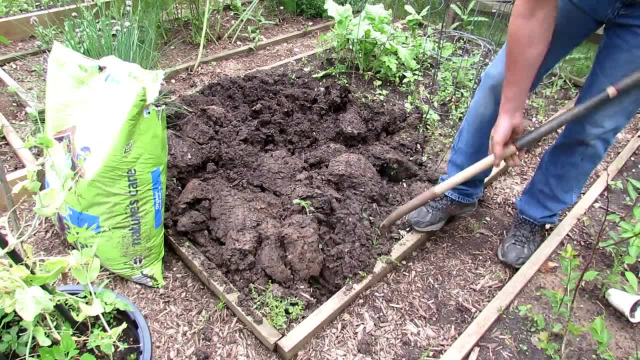 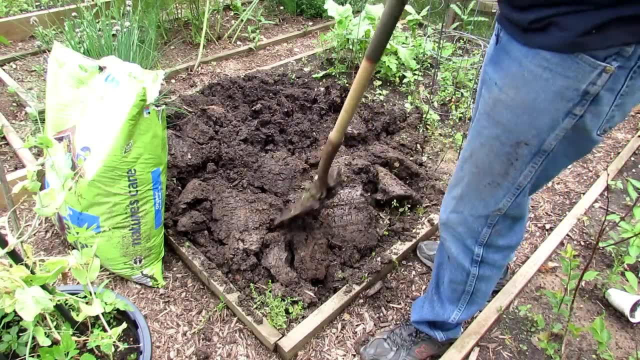 But most of the time you're going to have soil that might be too sandy, maybe a lot of clay, So you're going to want to add in some bag product And I'll talk about what to buy, But in a 4 foot by 4 foot space. 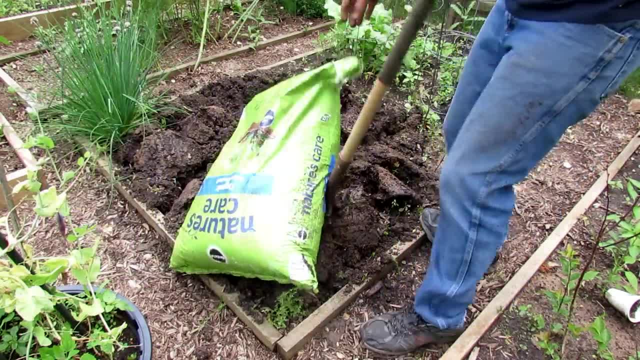 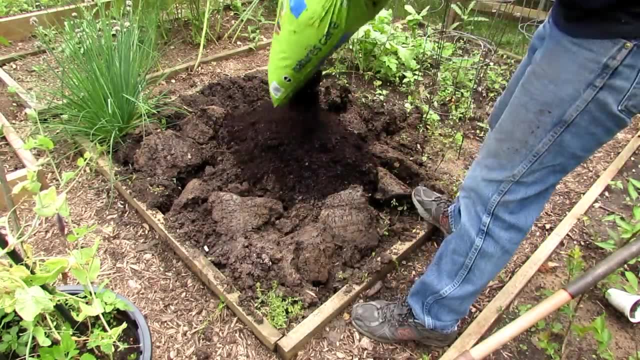 you want to have about 2 to 3 cubic feet of material that goes into here. This is 1.5, so you might need two bags of this, But it's about 2 to 3 cubic feet of some bag material. 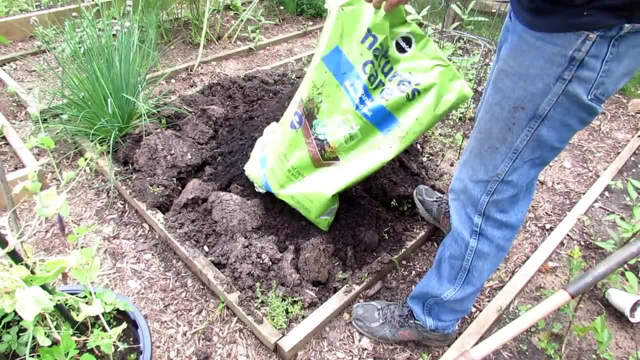 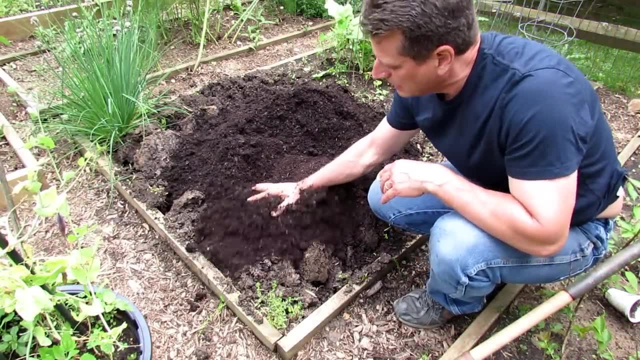 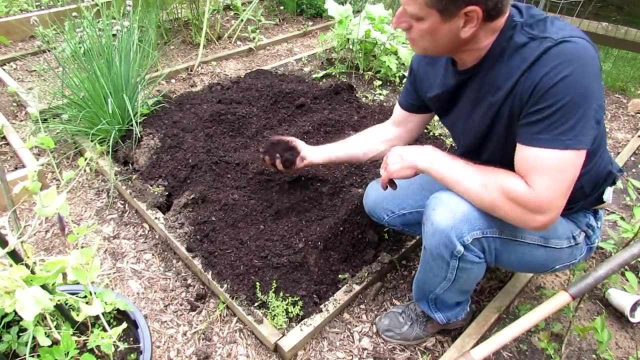 And you can use garden soil, You can use raised bed soil, You don't have to use potting mix or anything really expensive. So this is 1.5 cubic feet And you would just spread it out over the top. Now this is a completely different material than my earth soil. 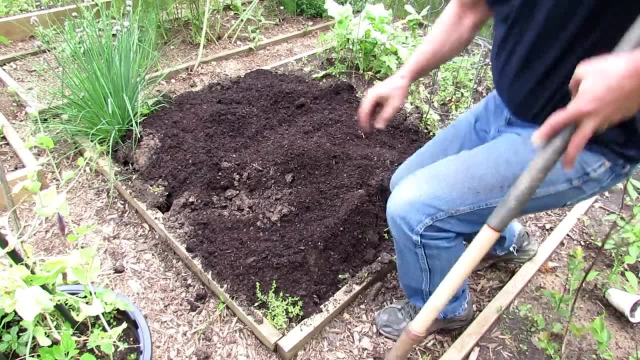 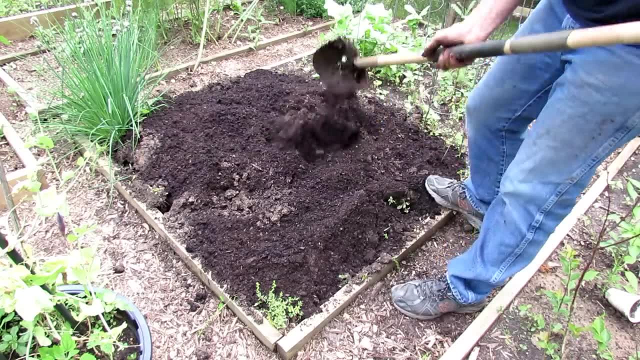 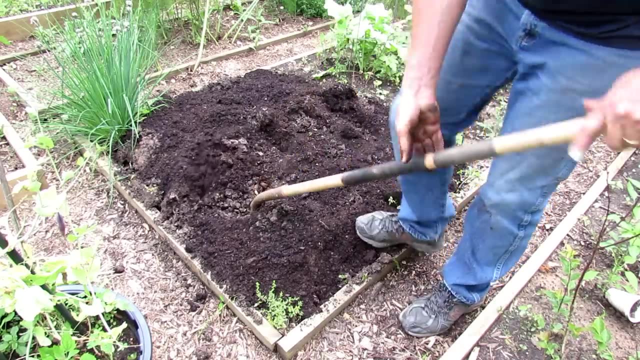 So you want to spread it out just like that And then go turn it over and chop it up. And the reason you want to do that is you want to mix it up nicely, because if you have layers of different soils, different products, when it rains it could be problematic. 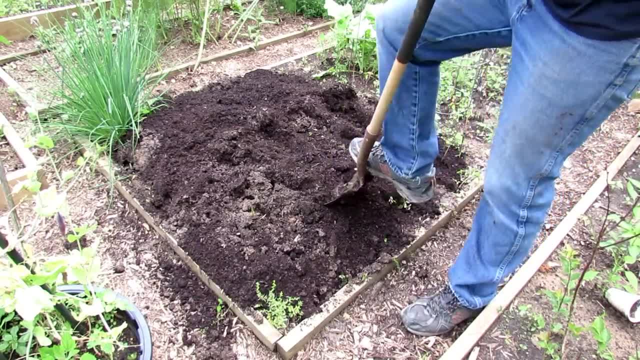 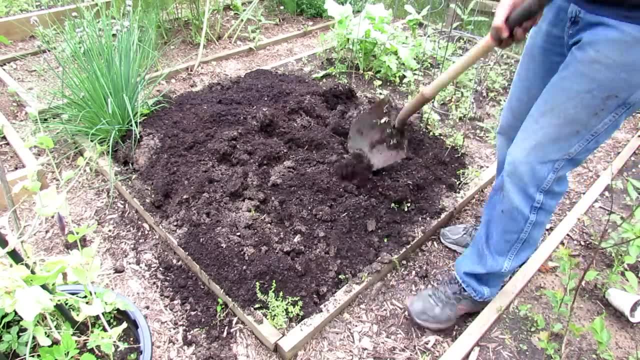 We're not going to fertilize this whole space. I'm going to show you how to fertilize just the planting hole of the plants. It'll save you some money. But you go ahead, You turn it over All just like that. 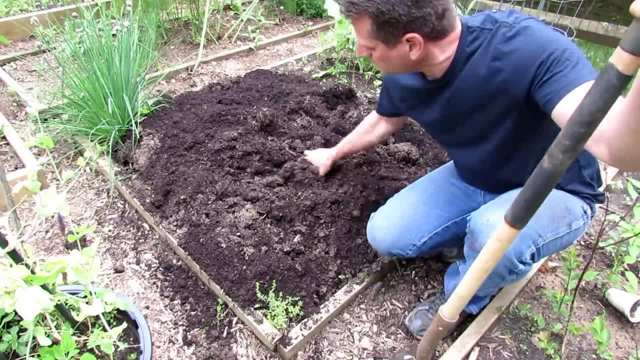 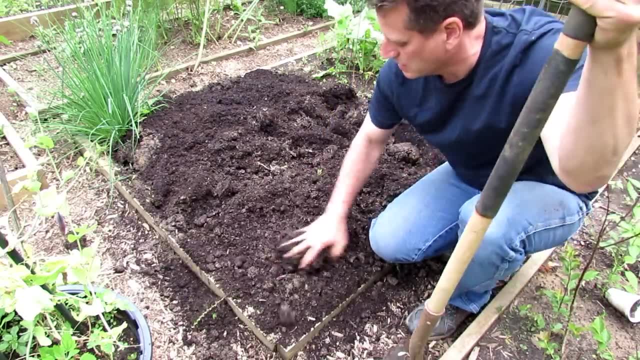 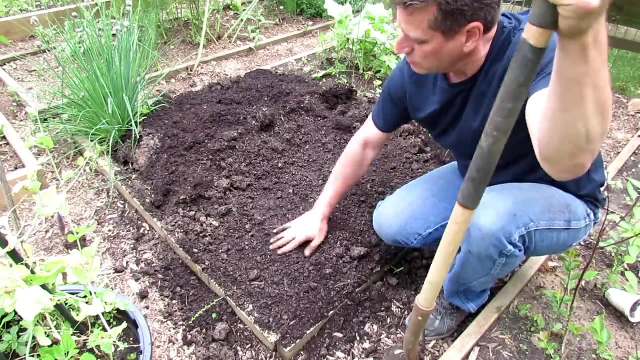 And I actually then like to get my hand in there and really mix it up, Break up the clumps And get your new space set up. Now I'm recommending you can just go ahead and do this in the ground. When you're doing it in the ground, you don't have the raised bed edges. 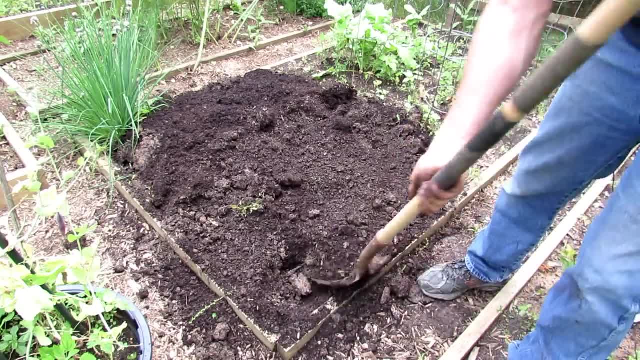 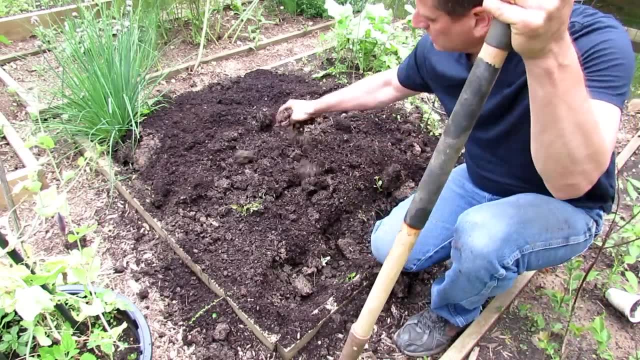 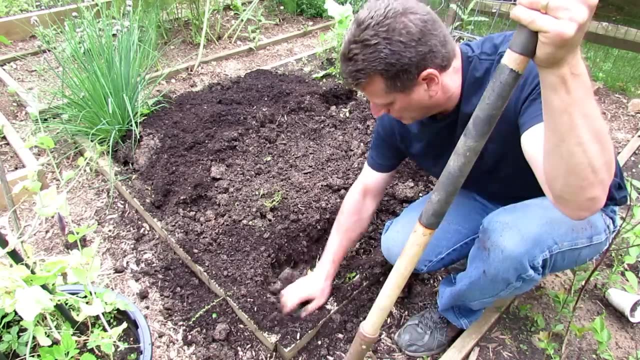 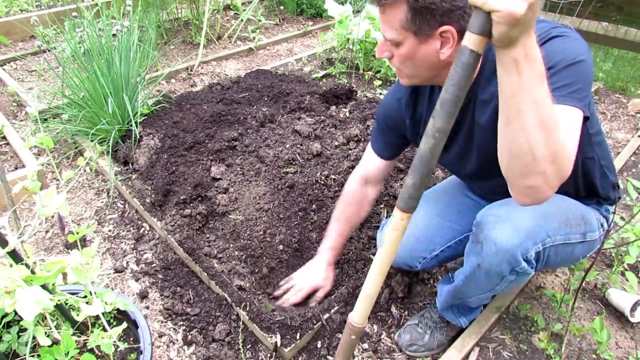 So go ahead and just dig a trench around the whole space, Just like that. Take out the clumps, Break it up And you would do that all the way around your space. That will let water run off to here. You can also water using the trench. 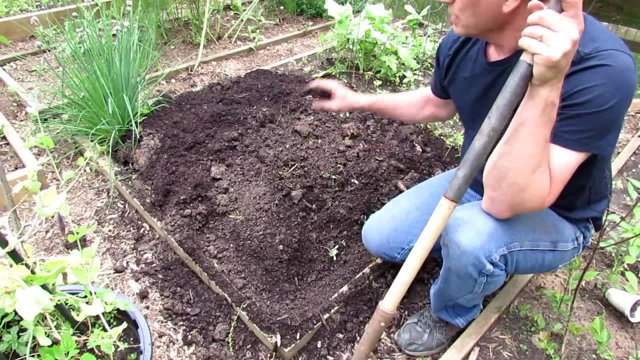 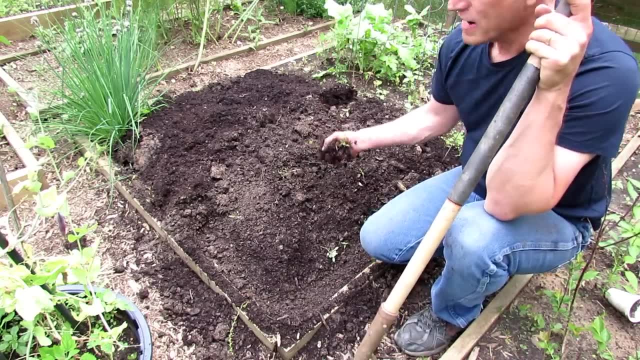 But this is the basic way you would set it up, Nothing fancy. I just encourage you to get started, Apply this basic principle And I'll show you how to do the rest. Okay, Let's get over to Nashville Tennessee, As I mentioned. welcome to Nashville Tennessee. 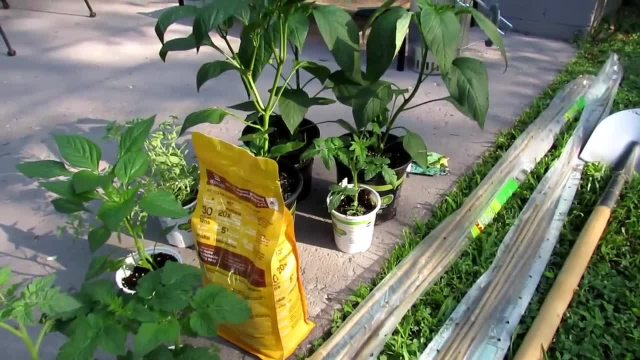 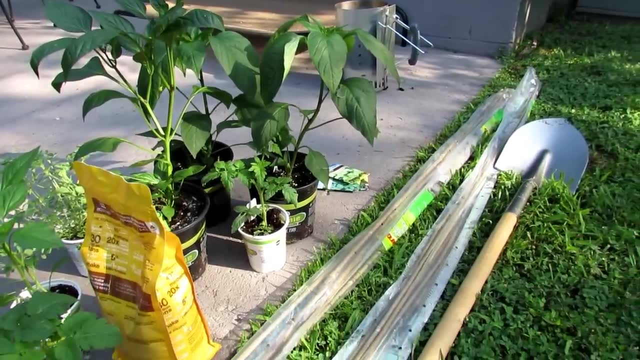 I am here visiting my son, Helping him get set up in his new place, And I always wanted to do a first dig, first plant garden. When I started the rusted garden, those beds are already made up, So I'm going to show you how to do the basic set up to get garden plants in that you buy as transplants. 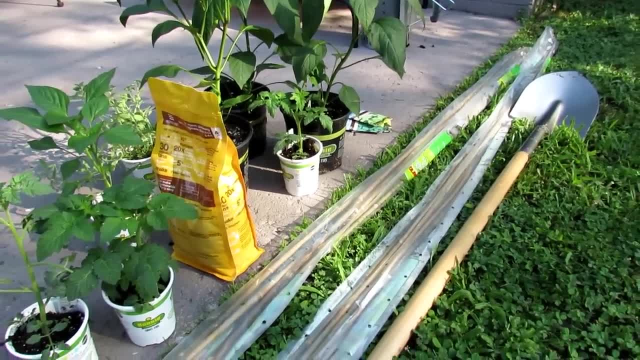 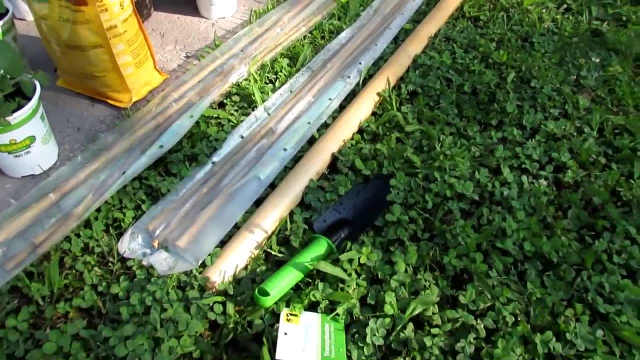 Certainly, you can use your own transplants, But this is really for the first time gardener- But you can adapt the principles as needed. You're going to need some basic items, What I like to call the small shovel, The big shovel. 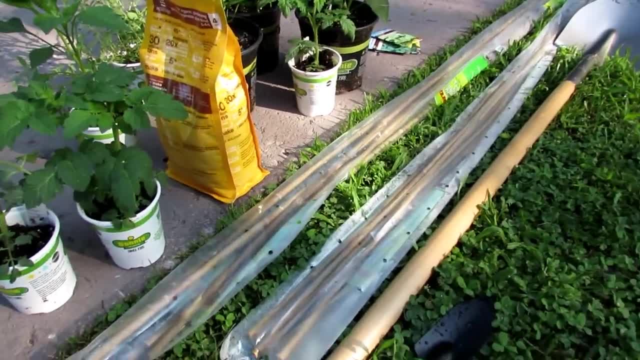 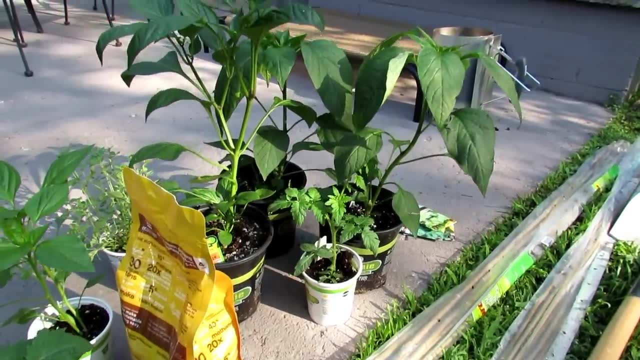 A couple of stakes, At least five feet tall. You're going to need your plants. I got these at Home Depot. The bigger ones are on sale right now, Three for $12.. Those are different kinds of bell peppers, Maybe a jalapeno. 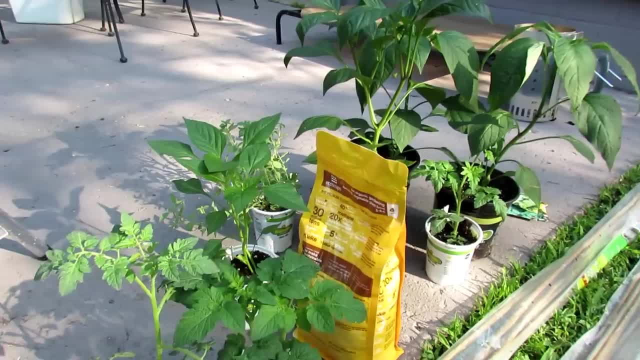 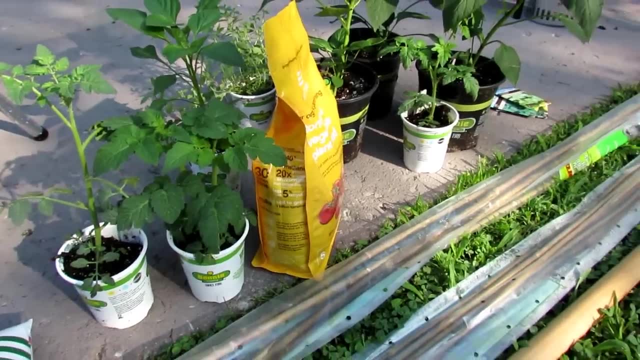 So I got three tomatoes, Four peppers Back. there is an oregano plant That's fine to buy as a transplant. You're going to need one bag of any organic fertilizer. Try and stay around a 5-5-5- N, P and K. 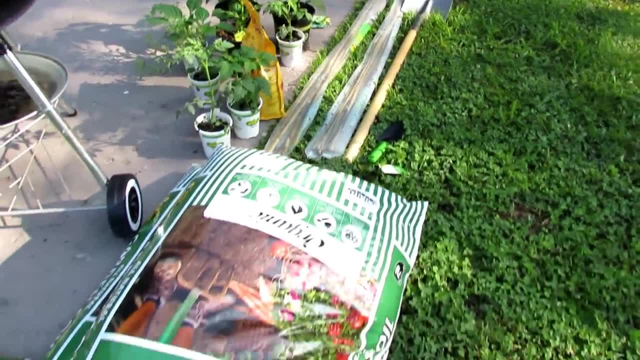 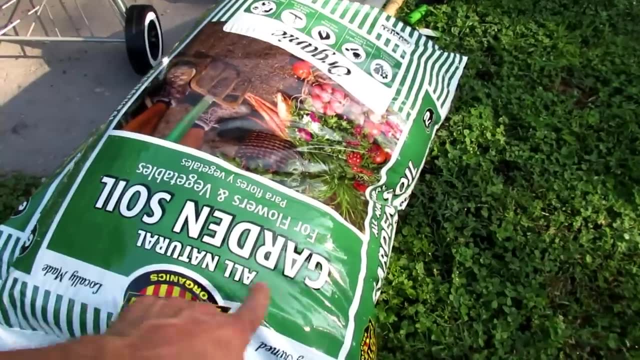 For this project I'm going to use two bags of garden soil, And I'll talk about that as we go along. You can get any kind of garden soil, And in this case definitely upside down, but it's garden soil, Because this is going to be all done right here in the ground. 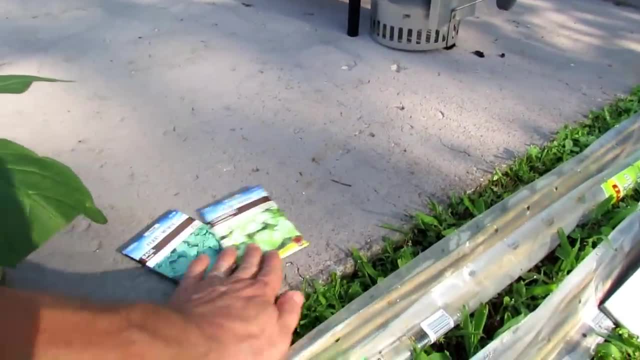 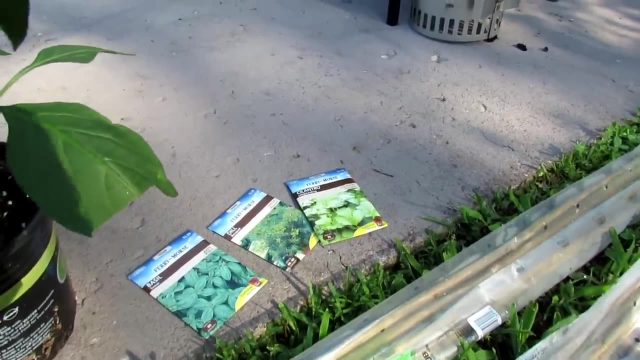 A couple of tips to save you money. When you go to the store you're going to see cilantro transplants, Dill transplants, Basil transplants. Don't buy those. Buy the seeds. These are annual plants in the United States in general. 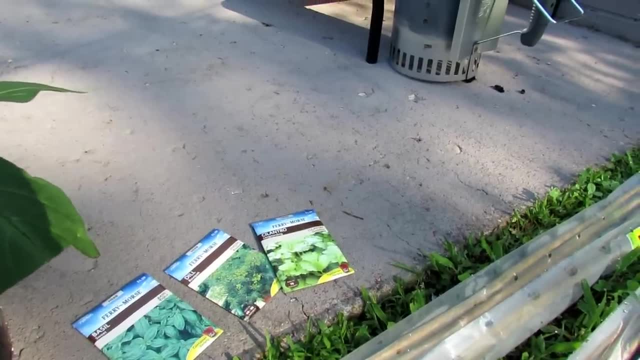 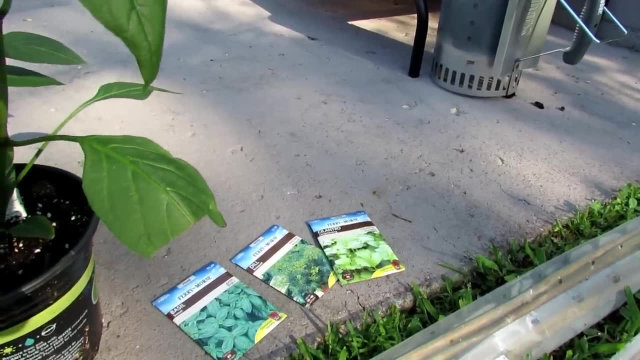 They grow in the warm weather, Although cilantro can grow nicely in the cool weather. But they all grow to grow flowers and reseed. So when you're buying them in the stores you're paying $3 a plant. They're at a good size already. 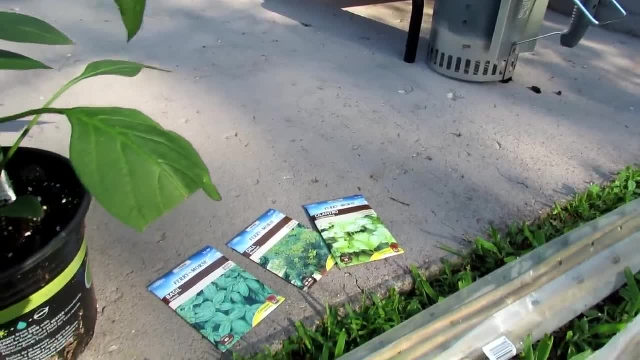 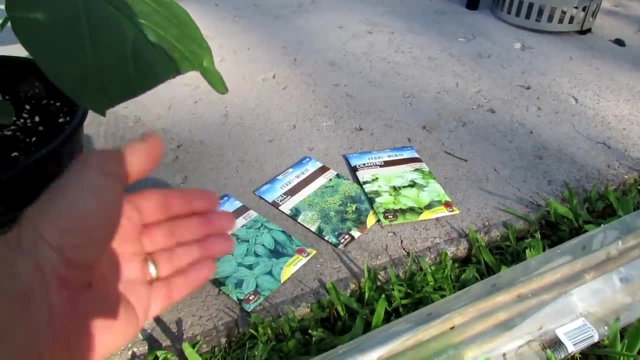 By the time you get them in the ground, they're good to go to flowering And they're not going To really produce for you. So start as seeds. They'll grow really quickly, And you can keep doing this over and over again. 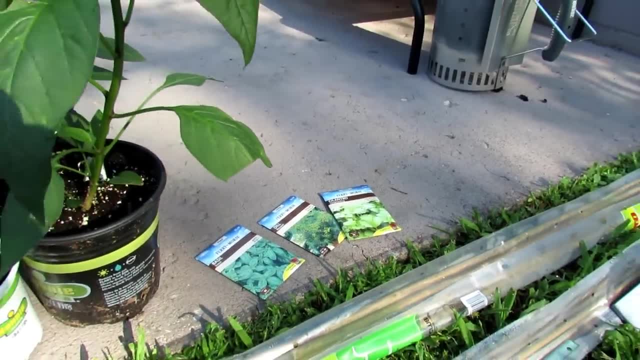 Because there's so many seeds in there. It'll save you a lot of money. You will get tons of basil, Tons of dill And tons of cilantro. Now let me go over to this space here. It's about 8 in the morning. 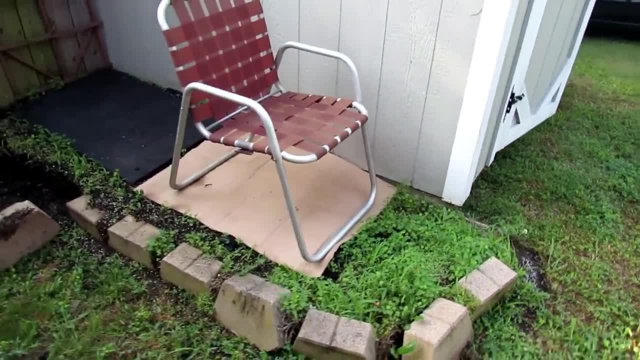 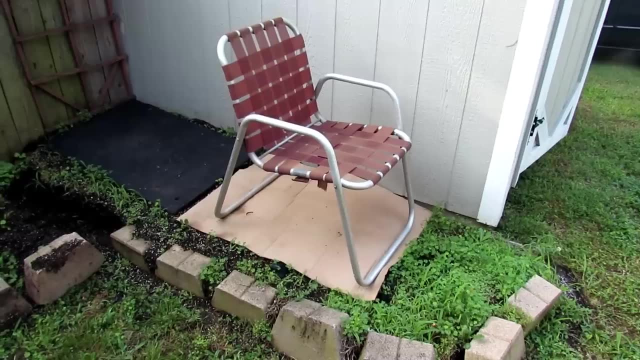 It looks like the previous owners tried having a garden here, So I'm going to assume that this gets the amount of light that it needs. And what's the right amount of light? Minimum, Minimum, Minimum, Yeah right, That means, is this going directly to your plant? 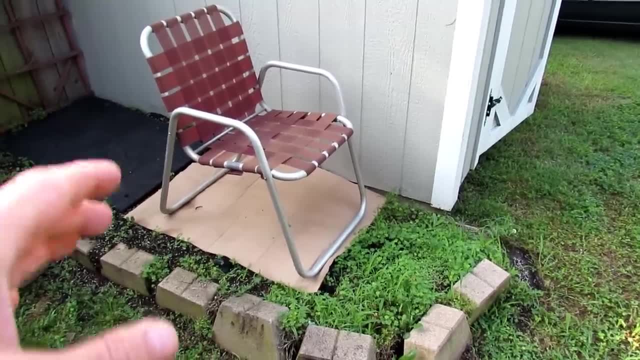 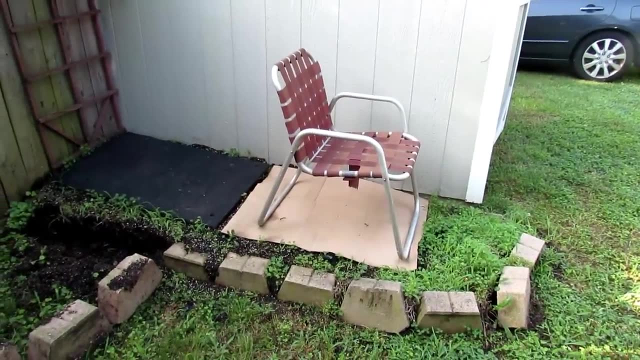 Right, Right. Well, you're at a full sun. That means the sun is going directly from the sky, directly to your plant. Not just bright light, but direct sun. And the way that you figure this out is to check out the areas before you plant. 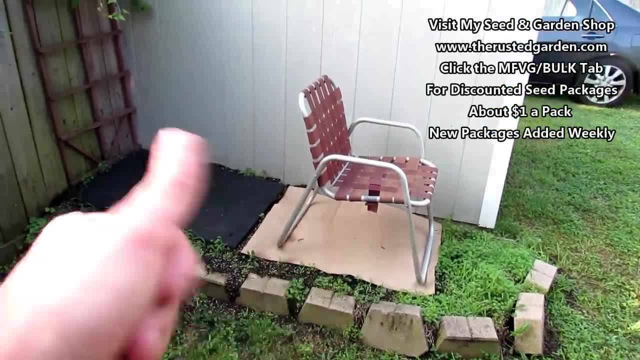 So you come out at 8 am And you see where the sun is. The sun is over here to my left, And I already know because I did this yesterday- And then you come out at like 10,, 12,, 2 pm. 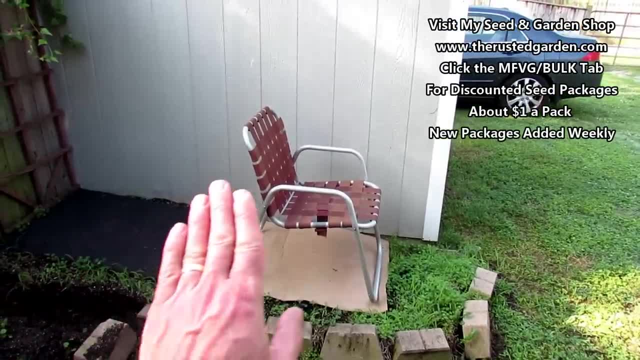 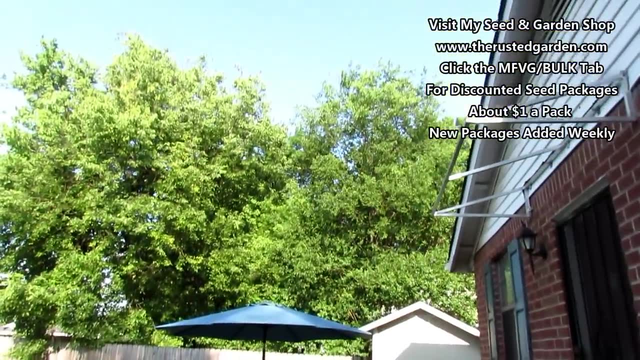 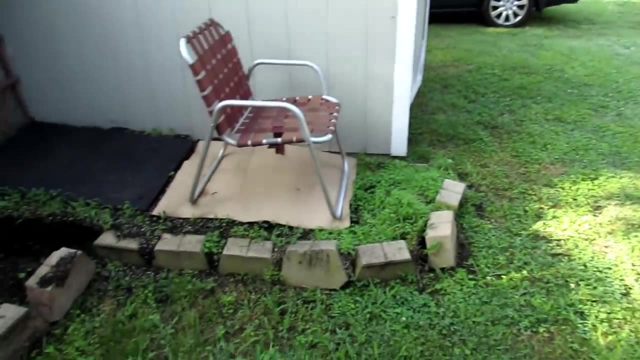 4 pm And you see where it tracks. And the sun here tracks from the left all the way over to the right- I'm going to slowly go up here- and it ends up over those trees, so plenty of light comes straight down from there right into this space. now the other tip. 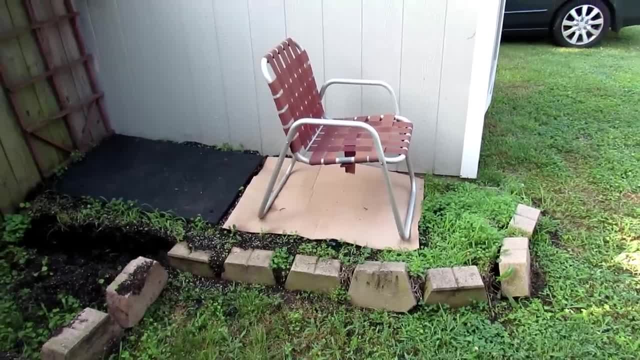 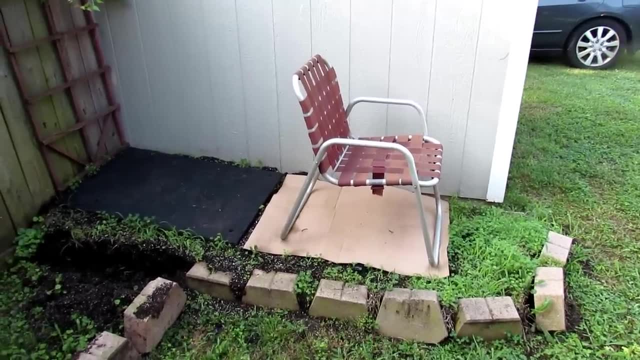 is is when you're doing this. you sort of want to plan. you saw that the leaves are on the trees. you may have trees near you. you do this in the spring, before the leaves form. you think you have plenty of Sun. the leaves come, block the Sun from. 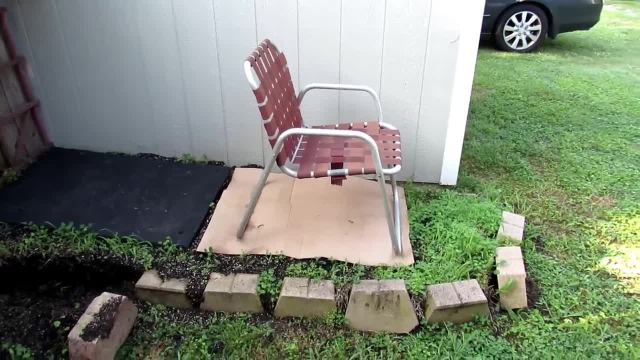 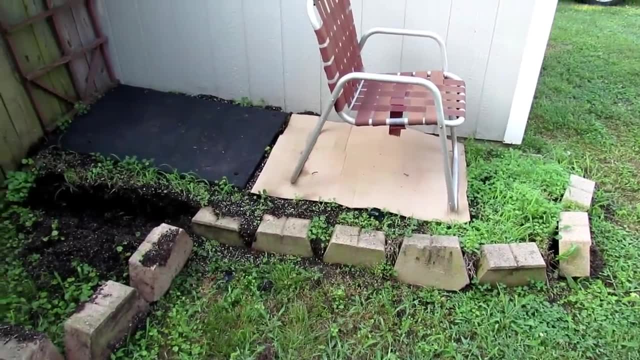 your garden, so you have to take that into account too. now, the other thing that they're doing here is they've raised up the ground a little bit. there's a lot of stone around here, so we're going to go with raising this up a little bit, and I've already repurposed this space. I want to talk about the size. 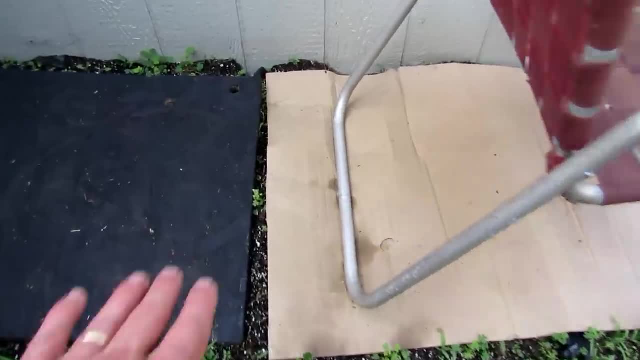 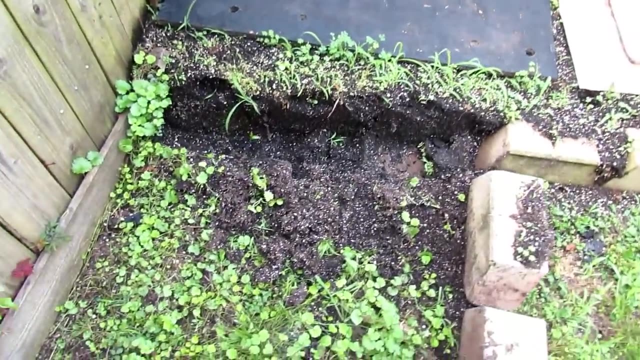 now, if we come up to here and we step right at the edge, you can easily reach in and get to what you need. sometimes people will use a corner. they'll dig it way out here and then, once you dig it way out here, if you try to reach there, 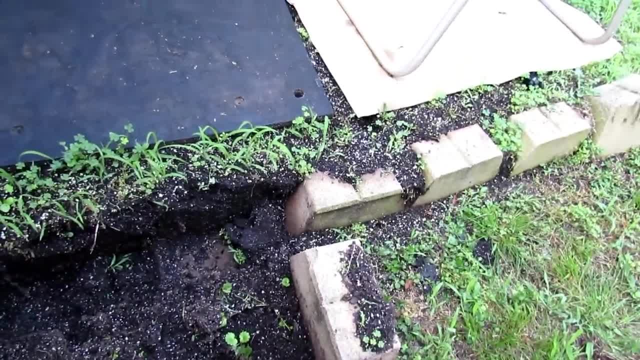 if it went all the way over that way. you can't get in this way the bait. the bed is raised, you don't see the leaves coming down from the trees and you can't step in it. you can put all your resources right in here and you can. 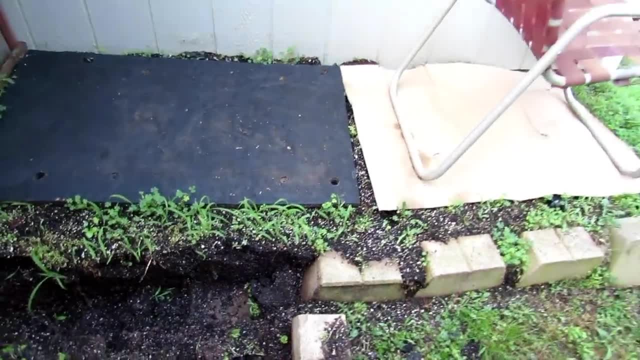 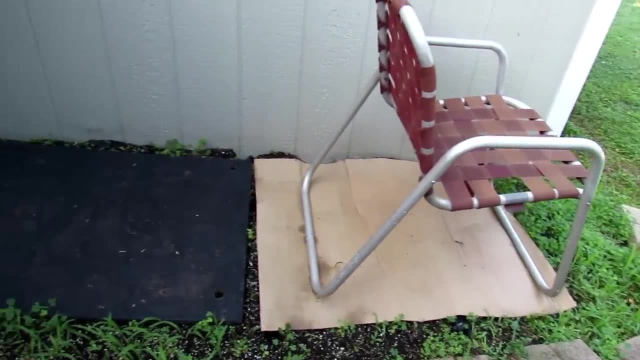 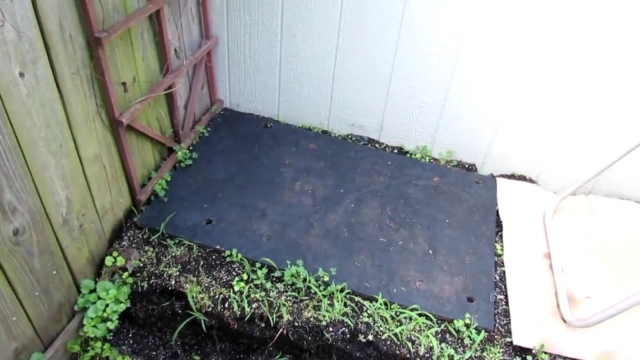 tend your garden without walking where the plant roots are growing. about two weeks ago, my son put down some cardboard. you can cover your space up, let it block out the light. it'll die. you won't have that many weeds and then you can go ahead and turn your soil under. so we're going to do this a couple of ways now. 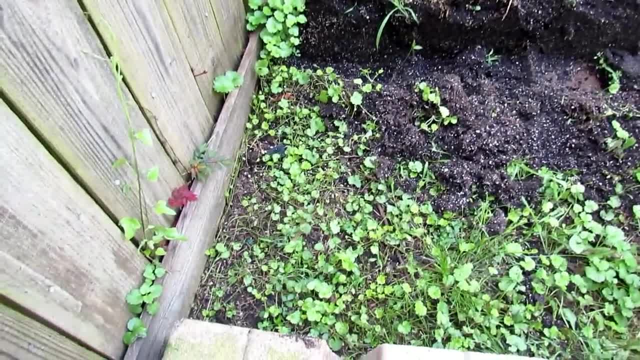 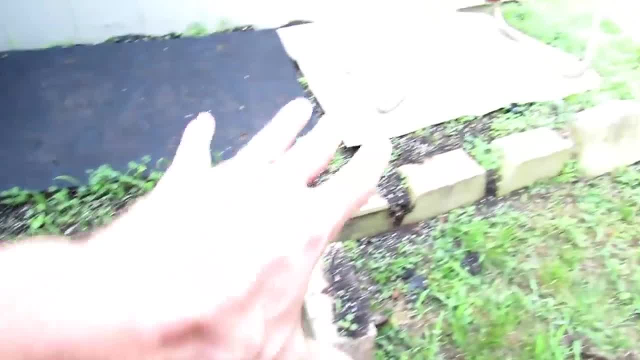 certainly right here. I could pull out some of the greens in there, get rid of them, turn the earth over with a spade, but I'm going to actually drop the cardboard there right on top of here and then kind of pull this dirt on top, put in the extra garden. so I'll show. 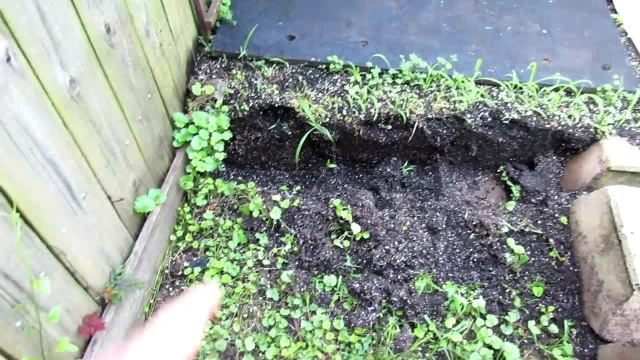 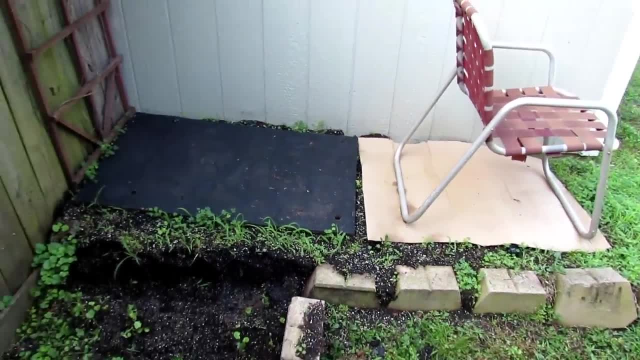 you how I do it. and then when we plant- because this is the first garden, we're going to dig specific holes for the tomatoes and peppers and plant. that way, I'll show you all of those steps because it's really important. you can learn a lot from this video, all right, and then the final tip: use your imagination. a. 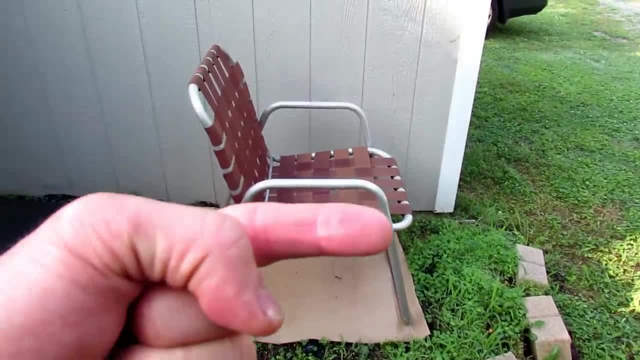 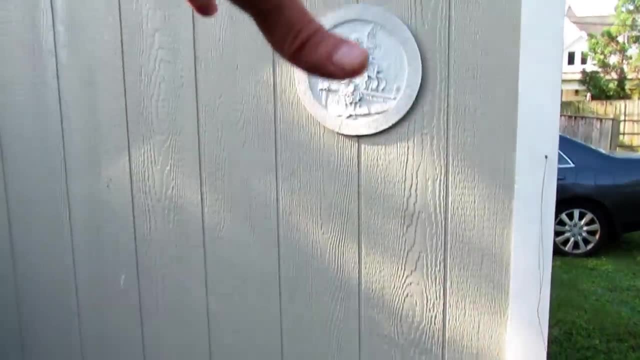 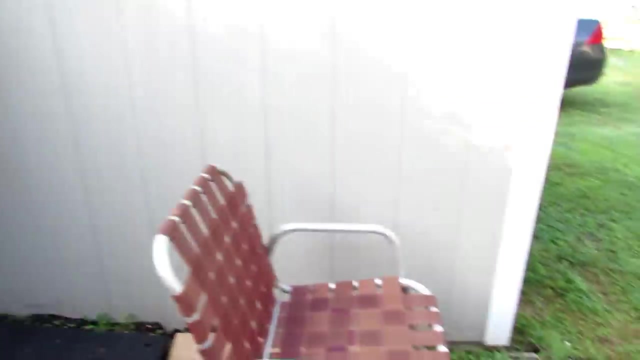 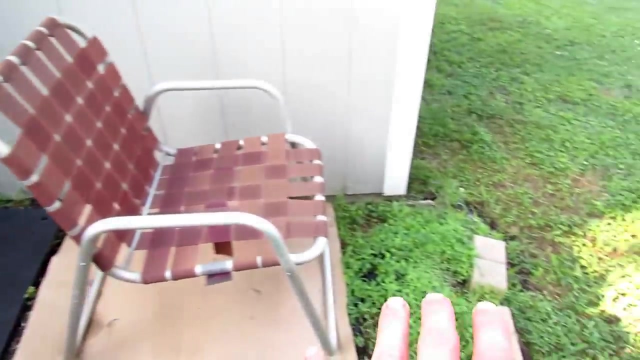 little bit because the Sun is over here most of the day. if we put the tomato plants right here and they grew six, eight feet here, what are they going to do? they're going to block the Sun from getting over here, so the smaller plants would go here. the bigger plants will go back here, so the peppers are. 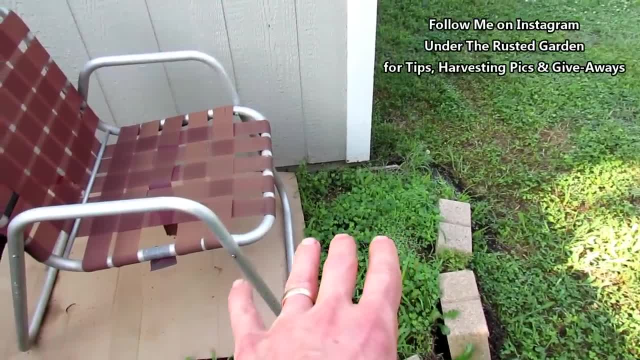 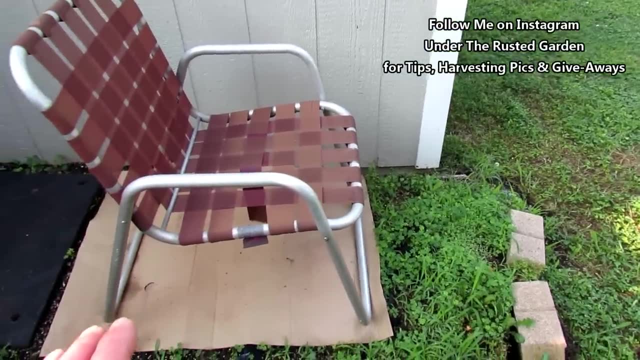 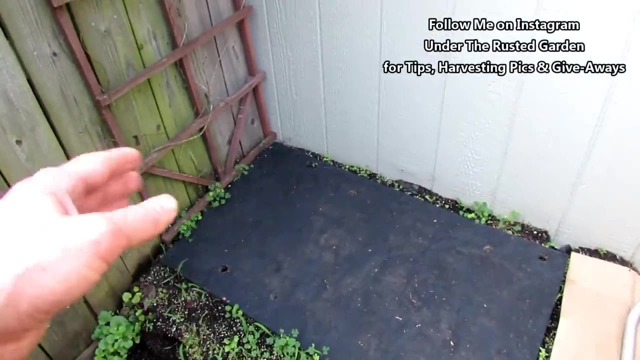 going to go right there because this area gets a little bit more Sun and they're going to stay low. they're probably get maybe three feet tall, if they're. you know, they're a bigger variety. I'm going to come back here. I'm going to put in the cilantro, the dill and the 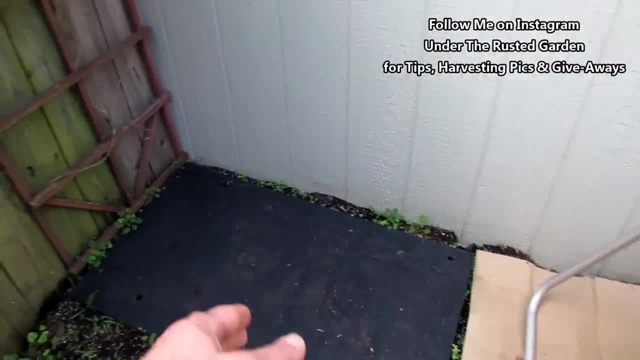 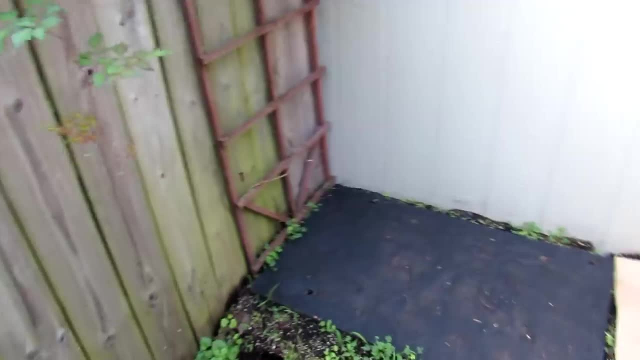 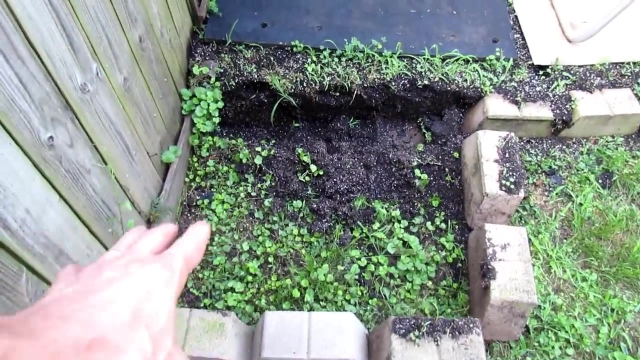 basil- actually basil, because it's a little smaller- cilantro and dill right in here, maybe a cucumber plant through here. I'm going to decide we'll also cut down all this greenery. and then, when I was checking to see where the Sun was coming from, this space gets a lot of Sun too, so I expanded out to here and at least two 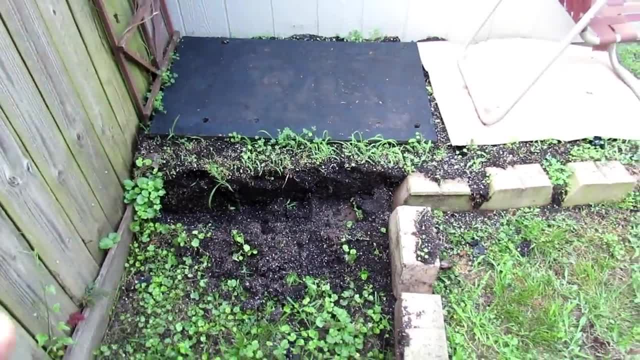 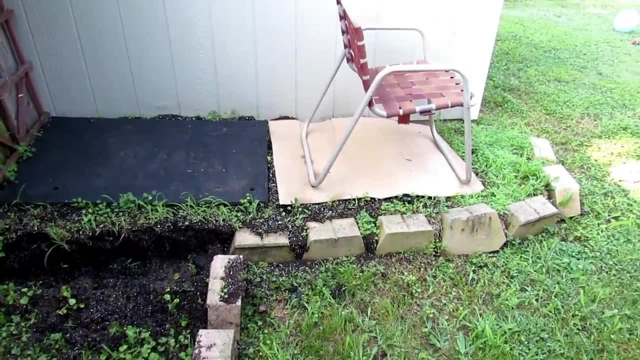 tomato plants will go in here. we can probably fit in three, but I'll get to all that. but you really want to pick the right area when you get started and keep in mind that if you have trees around you, make sure you check to see how the Sun tracks. 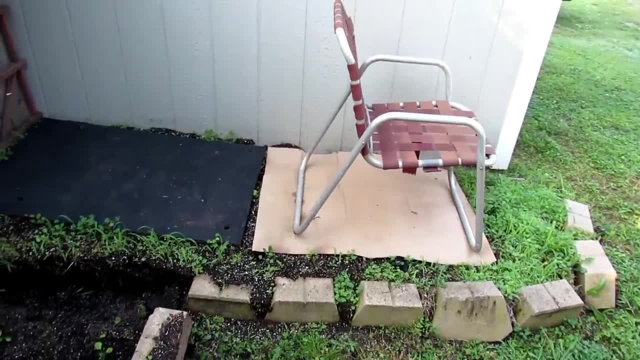 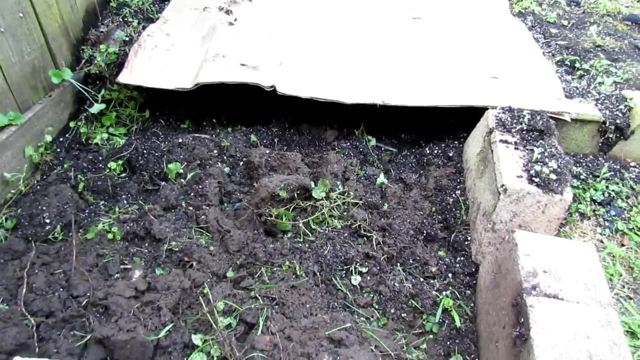 in your yard and onto your garden, imagining the trees have leaves. all right, let's get to the planting. a lot of times when you're thinking about gardening, you think you have to do a lot of digging and you don't have to do as much as you think, especially if you're preparing a little bit of a raised bed. 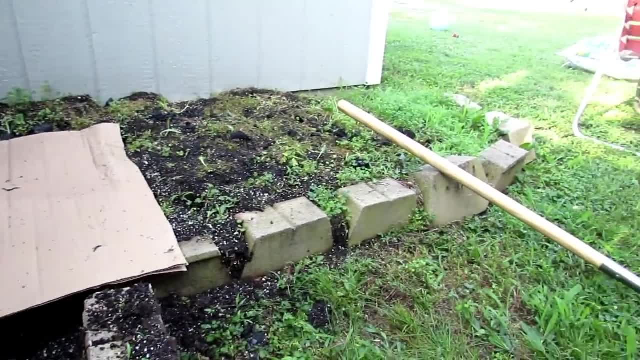 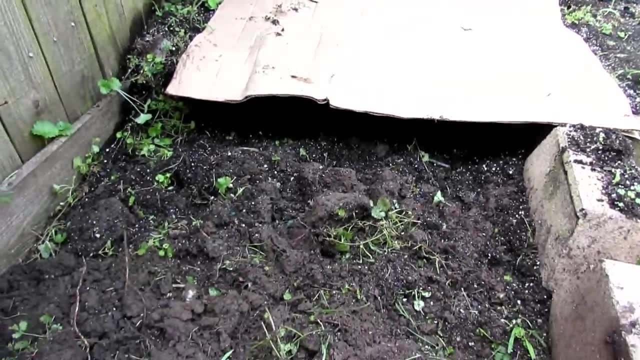 or just start with a small space just like this, and then you can get a lot of tomatoes, peppers, cucumbers and different vegetables and herbs you know to your kitchen table. so I just turned this space over. I was just going to leave it, but just turn it over a couple of. 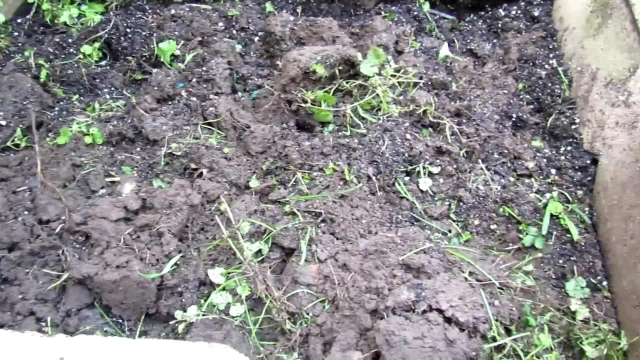 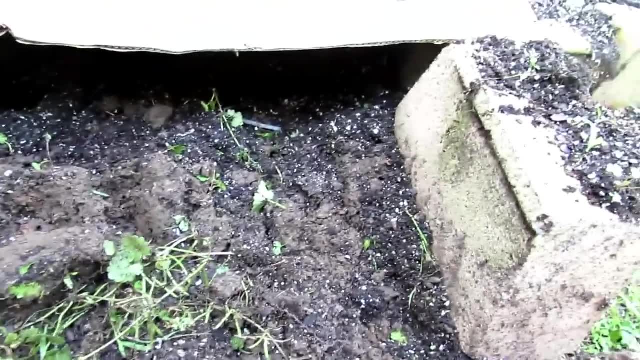 inches. you know three, four inches. turn the greenery over and you can see that their soil is naturally like this. it's a nice looking soil and they've already added a lot of different potting mix. you don't have to use potting mix in here. 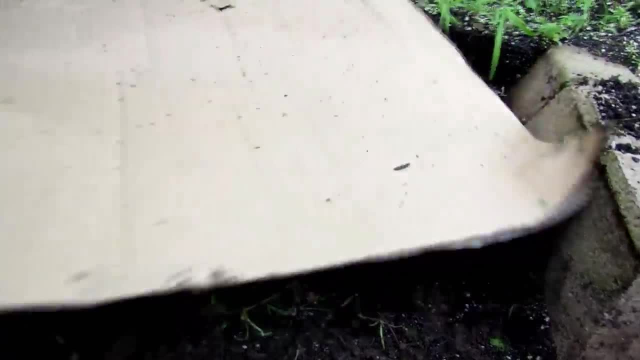 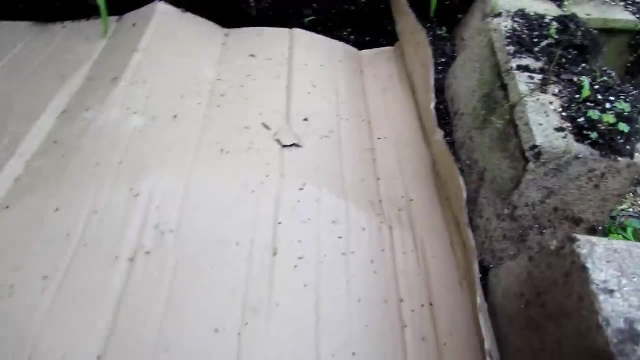 you're going to use the garden soil and the difference is garden soil will cost you less money when you go to Home Depot or places like that, and then you're just going to press and you can see all the black ants that have been living in here. if you do put down cardboard, a lot of insects will be under. 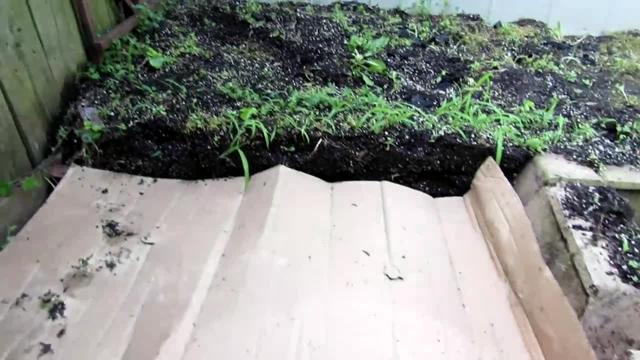 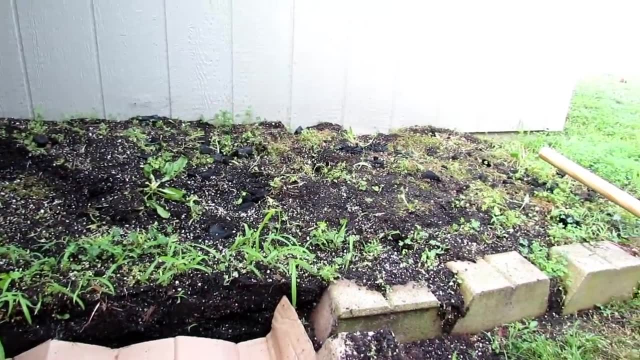 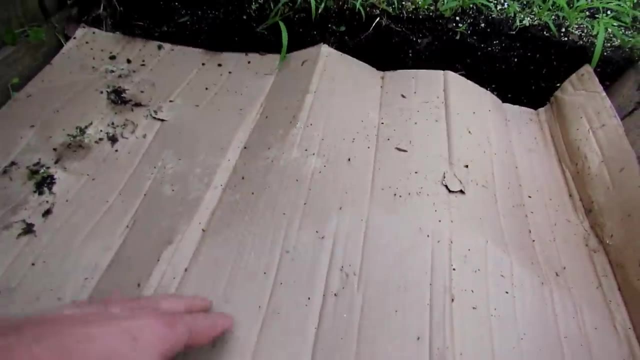 there. um, you know it's not a problem, once you disturb it they go away. but you could really go to a fresh area covered up with cardboard, wait it down. you know, wait four weeks, six weeks, it will kill out all the grass for you, make turning the ground over much easier. so we're going to actually just put this straight. 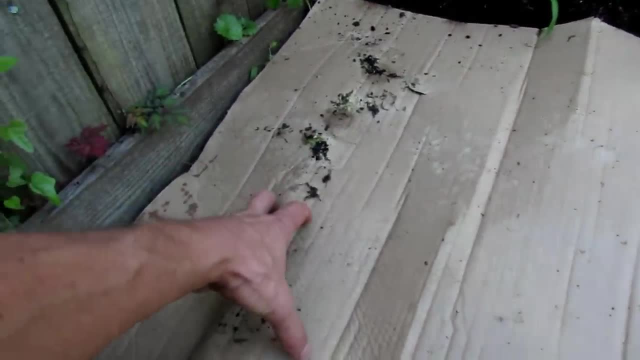 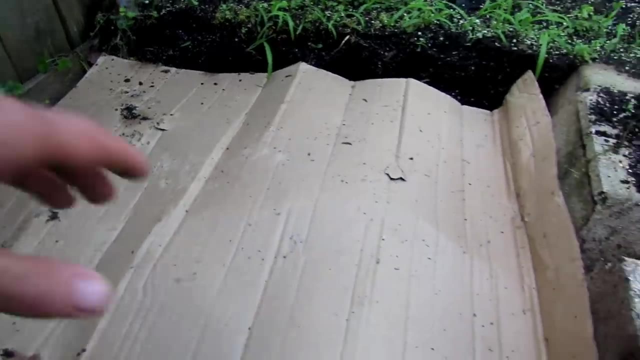 down, pull earth onto this, and then we'll do like a tomato right here. we're just going to dig a hole, put the resources there, put the plant in same thing with another one over there, and when this is wet, you can cut through this like nothing and it. 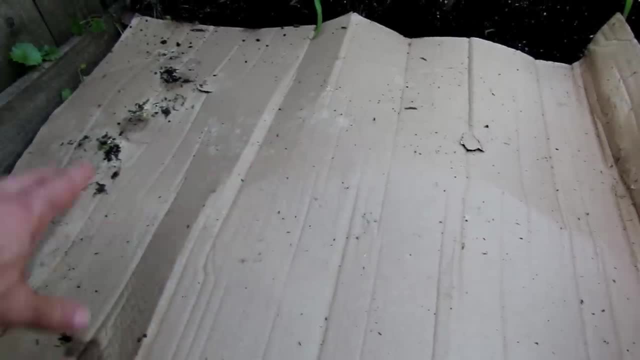 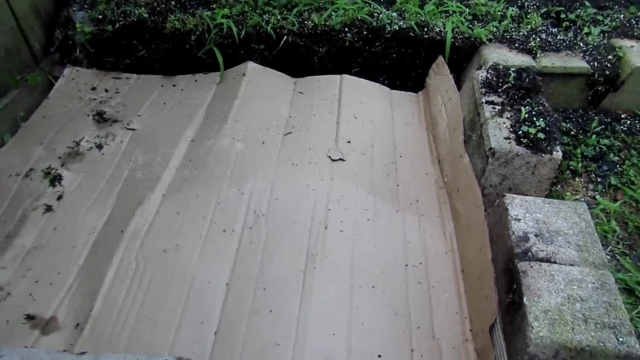 will suppress the weeds, it will decay, it will go into the earth. just make sure you use a basic cardboard. they usually have no chemicals or problems or anything like that- and then next year when you come back here, you'll turn over your ground and, you know, mix it together that way. so let me get to that. I moved the. 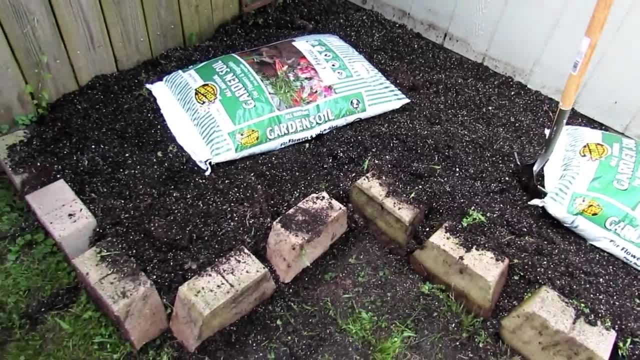 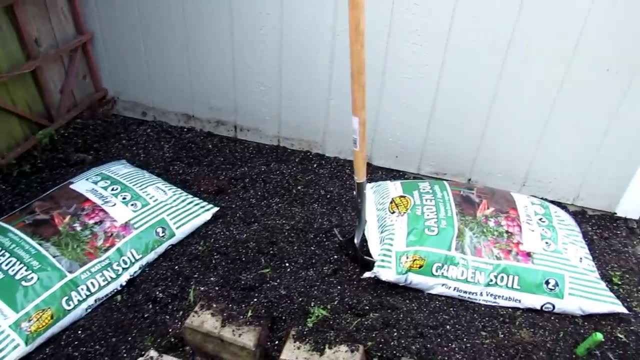 stones a little bit to space them out better. so this is technically a raised mound, raised bed and it was actually potting mix in there. all those white specks are perlite so it's really good soil in there. I just had to kind of fluff. 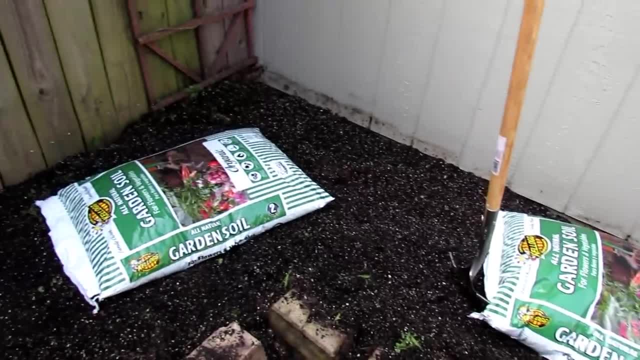 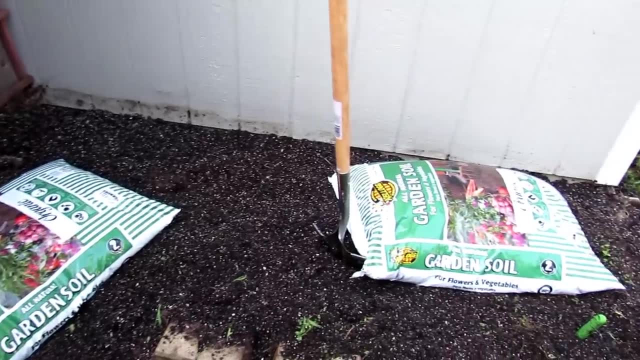 it up and spread it out. might not even need to put straight bags of the garden soil into there to raise it up. you might have to. so if they didn't put in all this really good container mix, you might have to drop in two bags as a two cubic foot bags maybe. 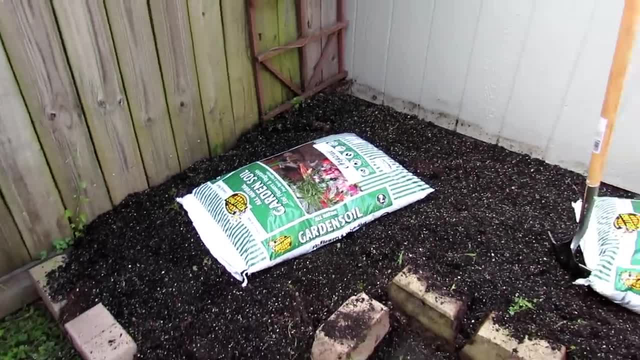 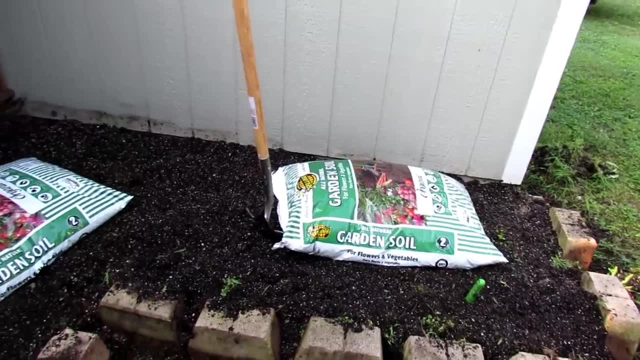 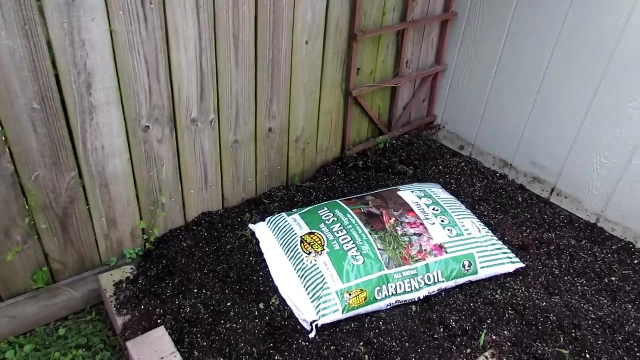 three bags into your garden area and just mix it all the way through. mix it in about four to six inches. you always want to blend any new garden soil you bring to your garden with the garden soil that's there and you just blend it together and that's so that when it rains, the water 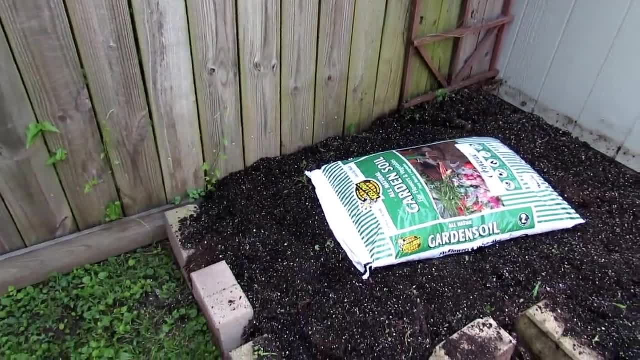 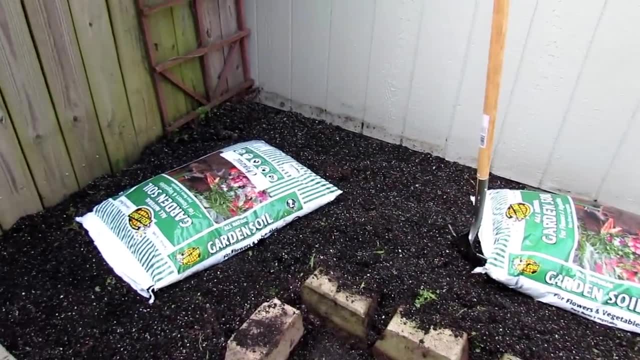 flows evenly from the top of the soil all the way down into the earth. sometimes, if you layer different soils, the water runs off in a funny way. so i'm going to use this garden soil- because there's so much there- for the specific planting of each plant, and i'll show you how to do that. 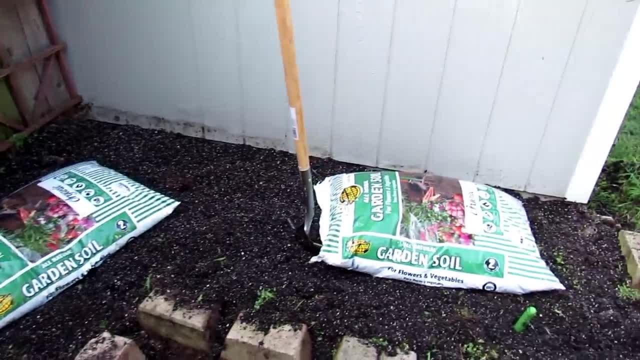 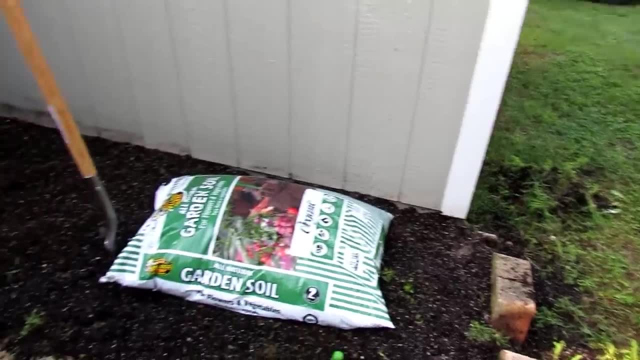 and that's again a way to conserve resources. weeding was really easy: just go and pull out any clumps that you feel like are best pulled out by hand. i just tossed them over there and then just turn the rest under. so okay, let's get to planting the peppers. so these are two. 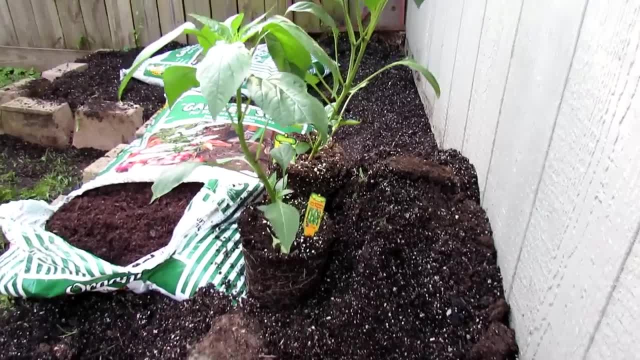 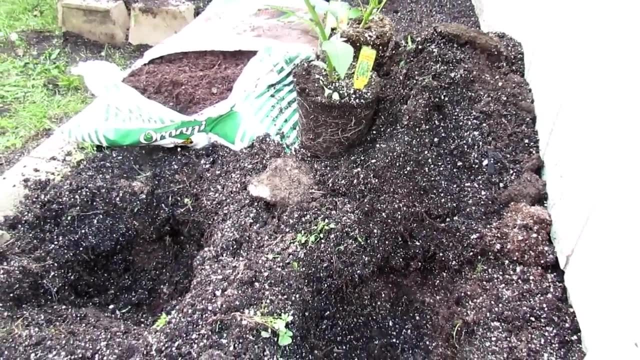 bell peppers that are gonna go in. actually, one of them is the jalapeno, the other one is an orange bell in the back and then behind there will be a green bell pepper and you can mix hot peppers and sweet peppers, peppers next to each other. they don't cross, pollinate for this year, creating, you know, a. 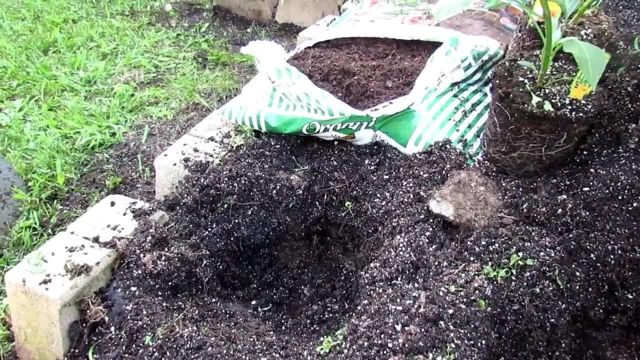 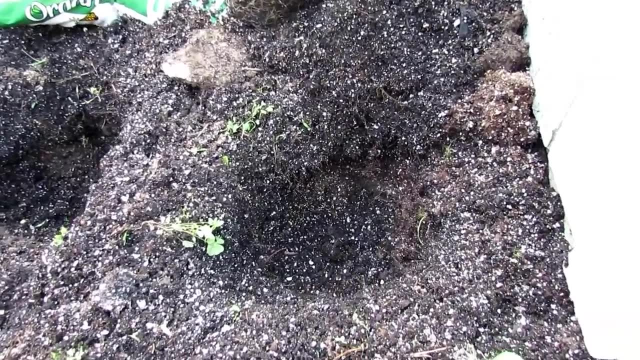 bell pepper that you're going to eat. that's going to be hot. that really comes for the seeds for the following planting. so feel free to plant sweet and hot peppers next to each other. so we dig a hole about that wide, eight inches deep, and as i got past the potting mix i got down. 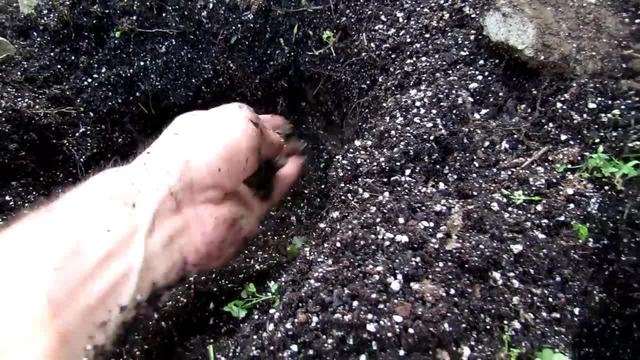 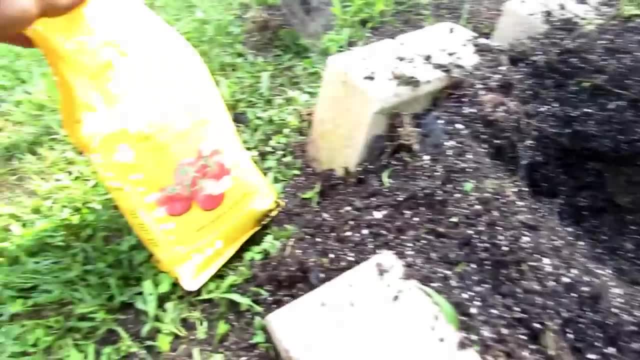 to the regular soil. it's kind of heavy, so that's what we're going to want: to loosen up. i also found a lot of stone, so that's why they are kind of raising the bed up. this is a 5, 4, 6 npk. 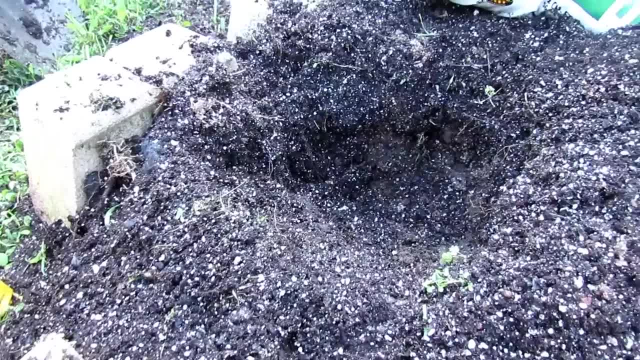 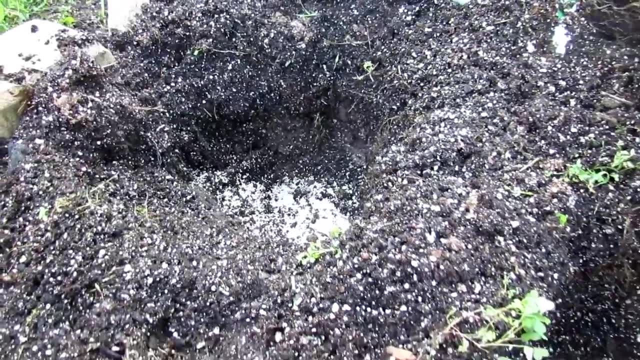 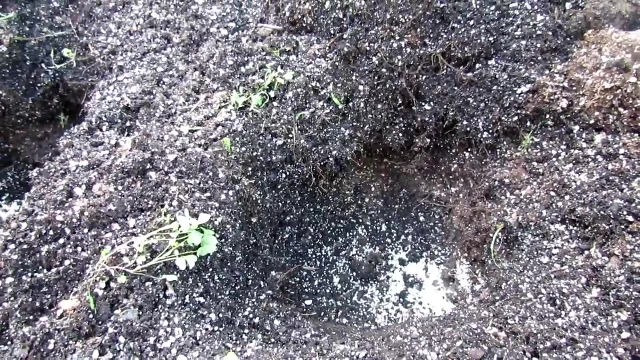 you really just want to stay around the 5, 5, 5. if some of the numbers are lower, that's perfectly fine. one tablespoon, two tablespoons. that will set up the depth of the hole for the root systems to grow into. and this is what you're really doing. is you're taking? 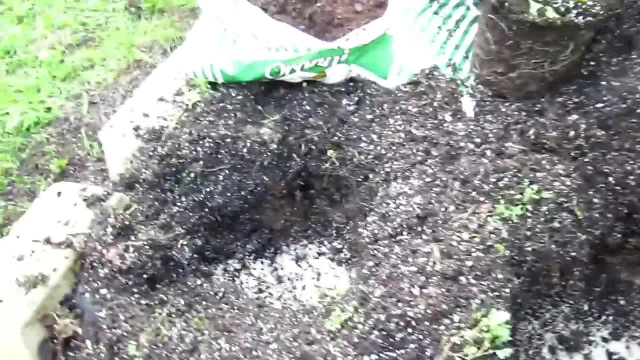 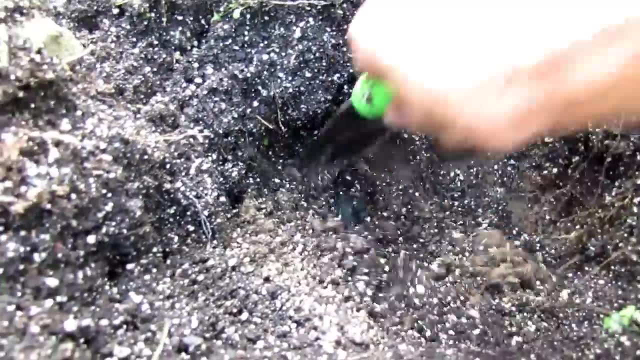 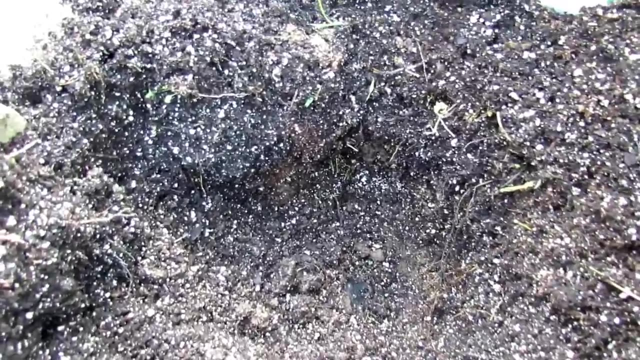 the time now to prepare the whole well and just get in there and then mix that into the top three inches or so, and this is where, because i have container mix, i could certainly bring that in. but if you had a heavier soil or needed to, here's the bag stuff. 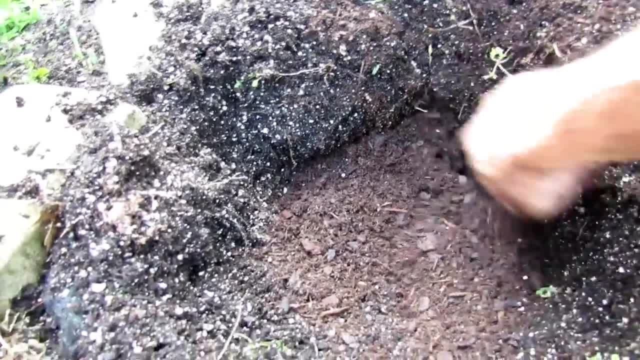 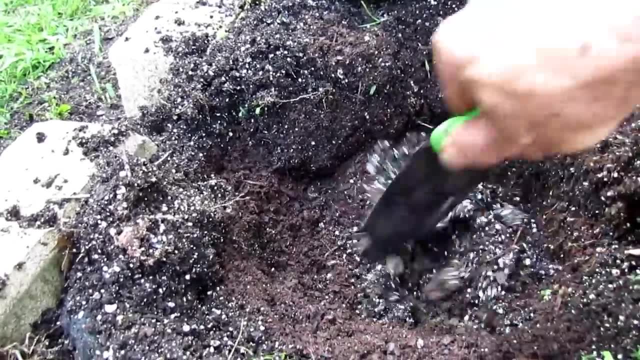 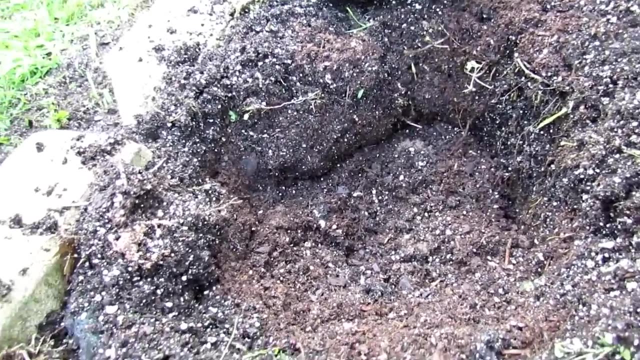 you're just going to pull that into there again. always mix your soil together, your earth soil, your bag products. just blend them nicely. and again, i'm doing this right handed, so you can see. next step is dropping the pepper. you can go to about here on the pepper plant. 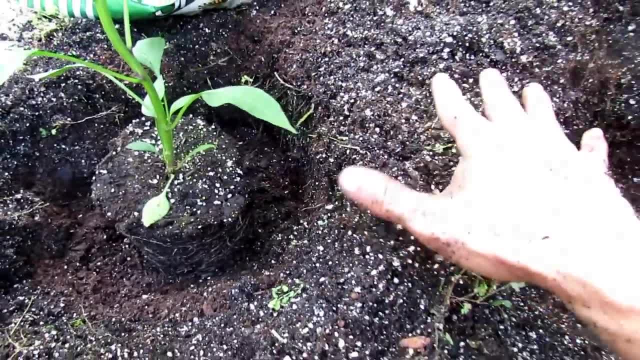 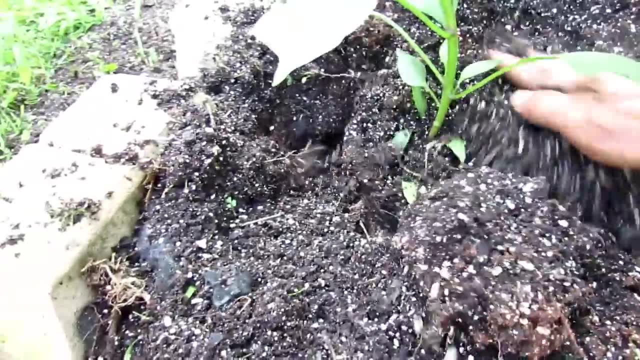 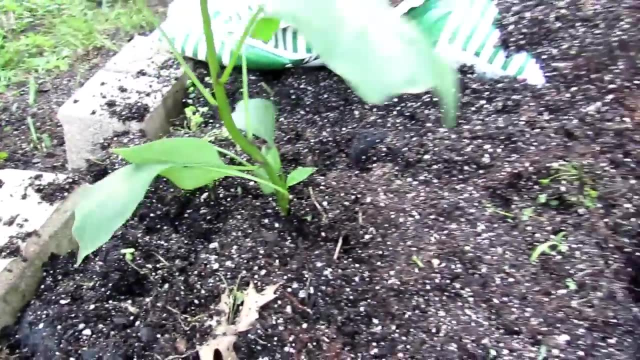 peppers will actually root out a little bit and the spacing we're giving them is one foot. i've done a lot of videos on the spacing of peppers and they can actually be planted a lot more closely together than you think. so that will actually set up that pepper plant, just like that. let me get to this. I'm setting it. 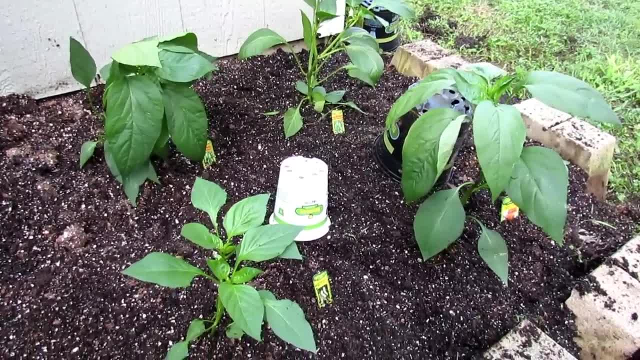 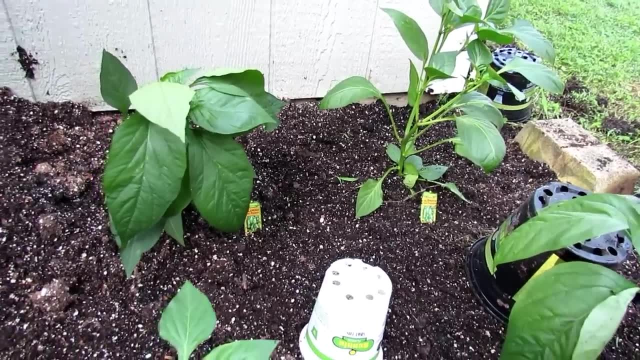 up the same way. the peppers are in about 12 inches to 18 inches apart and i actually thought that i got two green peppers. i mean one green pepper, but i actually got two jalapenos. so the peppers in the back are jalapenos. the peppers in the front are the orange bell on the right and the sweet banana. 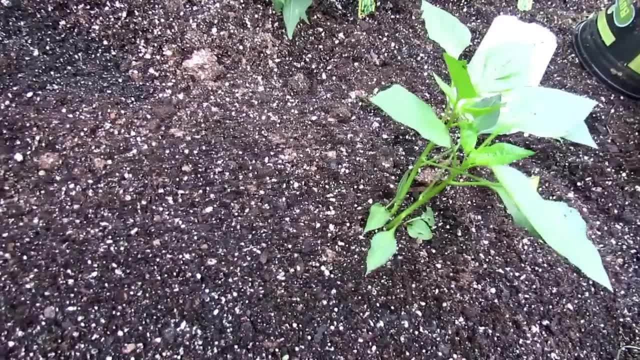 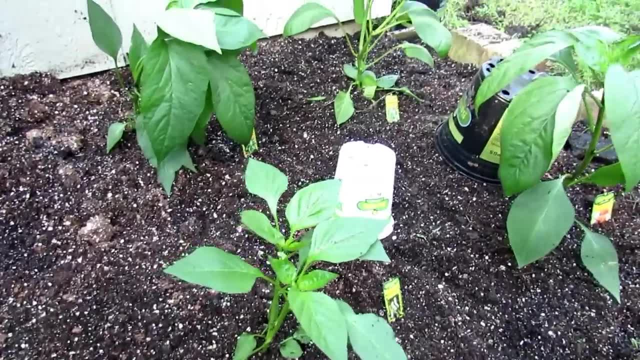 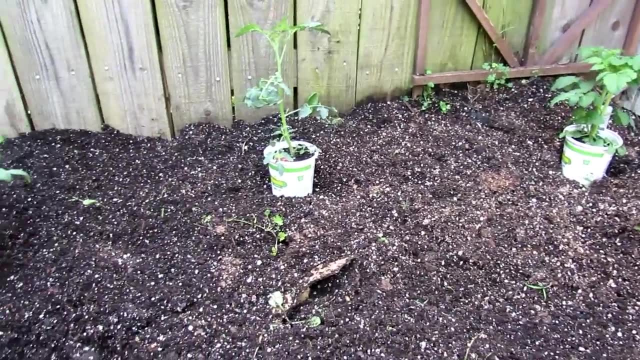 and you can see the sweet banana that i bought actually had two plants growing out of there. you can do that with peppers. you can put two plants actually in one space, so So they'll get a nice mix of sweet peppers and hot peppers Coming over here. I'm going to try and put in three tomatoes, and if you're just starting, 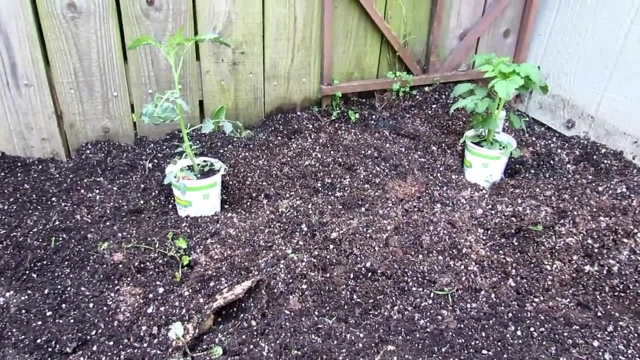 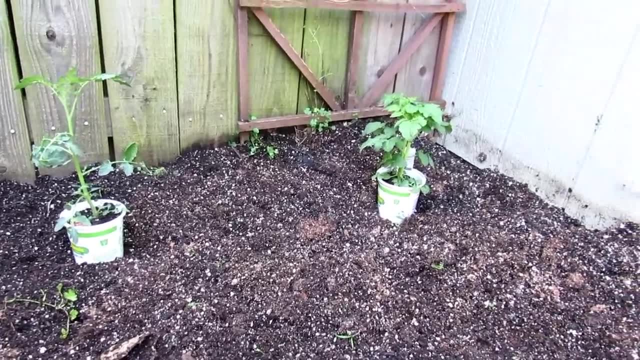 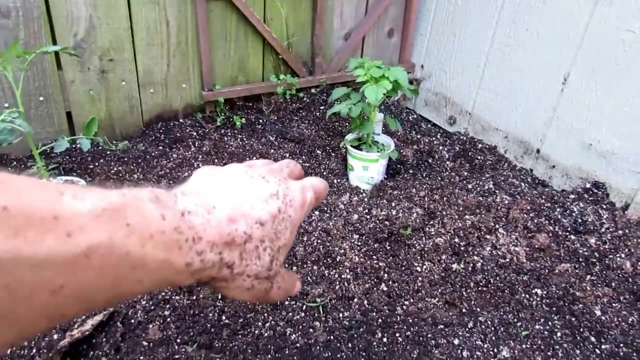 two would be fine. The two right there are cherry-type tomatoes. they're indeterminate varieties. Indeterminate varieties mean these tomatoes will grow until frost or disease takes them. So they're going to get six, seven, eight feet high. So if you're just getting started, probably one cherry tomato right in there and then 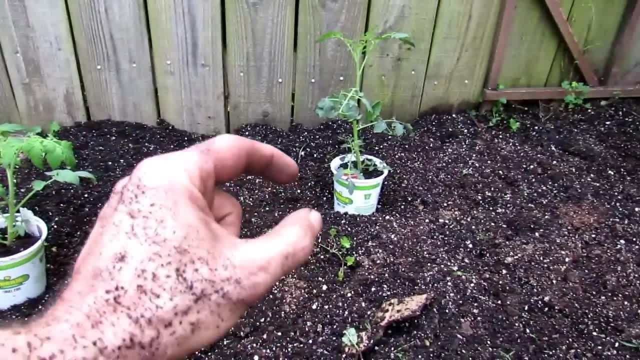 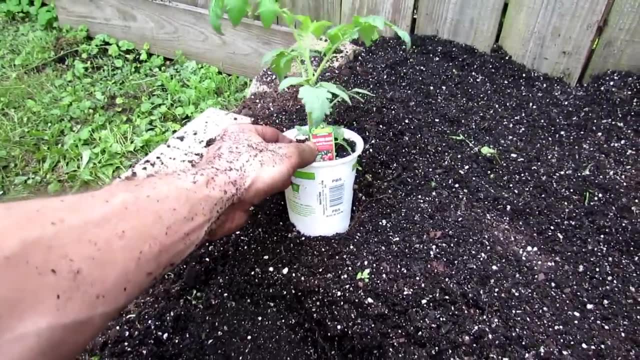 another indeterminate variety over there. Now what's the difference? The cherries are the small. you know cherry-type tomatoes you get in salads. This is an indeterminate variety also. It's good to grow as tall and it's a better boy. 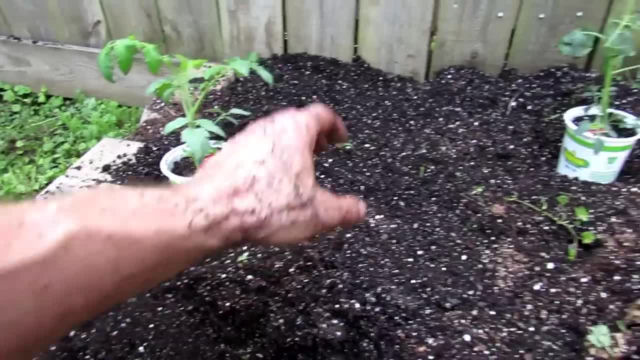 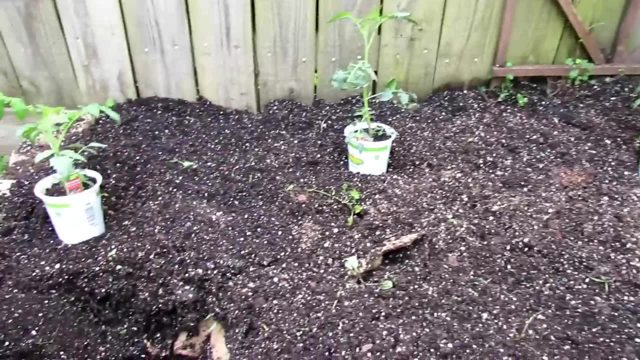 But these are about a little smaller than baseball size, more for slicing and that would go right there. So you would put one tomato there about two to three feet over another one there, But I'm going to space them out like this: 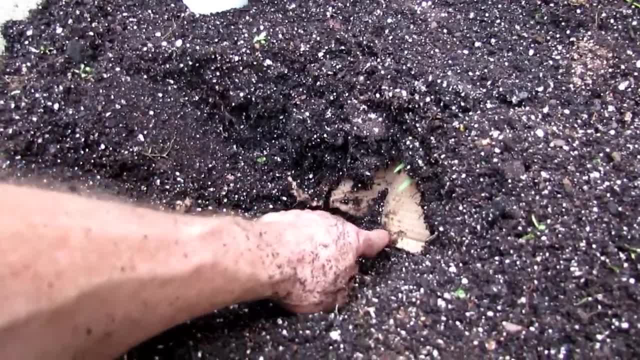 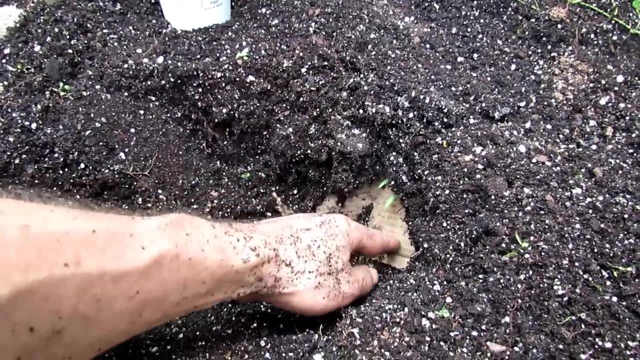 I wanted to show you the whole. So if you put cardboard down and then you put your purchase soil on top or other earth soil from me, Your yard, This will keep the weeds out. It's good at decay, But when I stuck the shovel in it just cuts real easily. 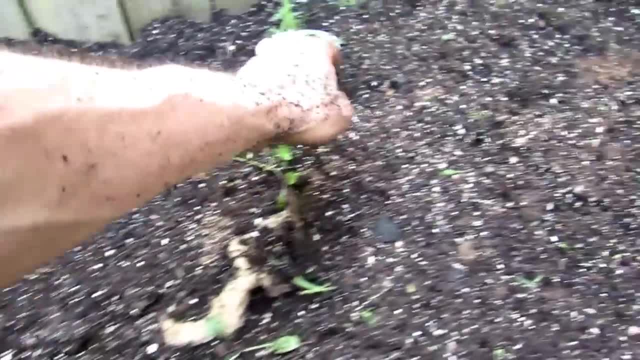 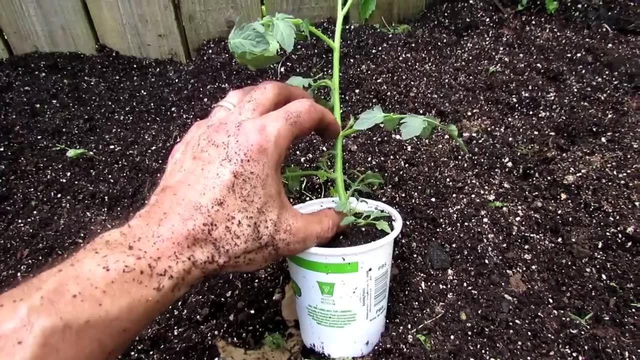 So I'm going to prepare this whole, just like I did with the peppers. When you plant a tomato, you can bury about a quarter of the stem, So these are going to look a little bit smaller in the hole and roots will actually come out. 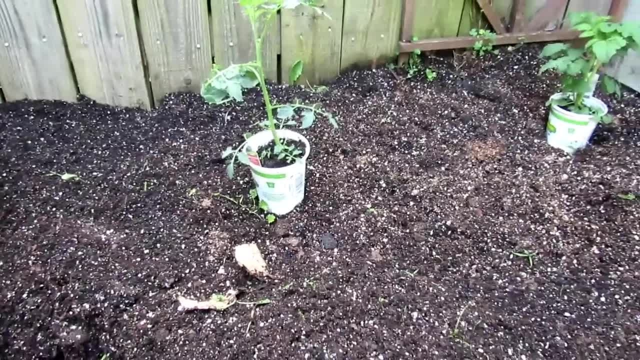 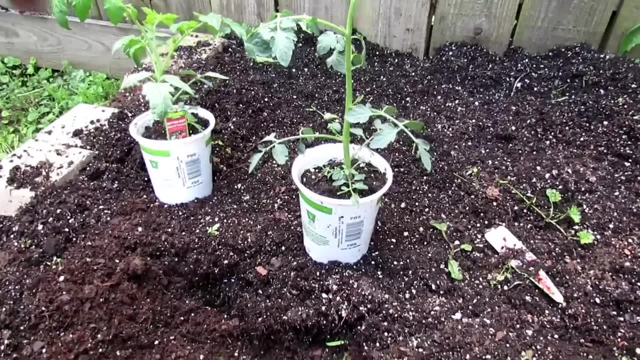 of here. So let me get the tomatoes in and then we'll get to top dressing, staking and then also seeding the cilantro, basil and dill right in here. You can check out my YouTube channel For more details on planting tomatoes, peppers and other vegetables. 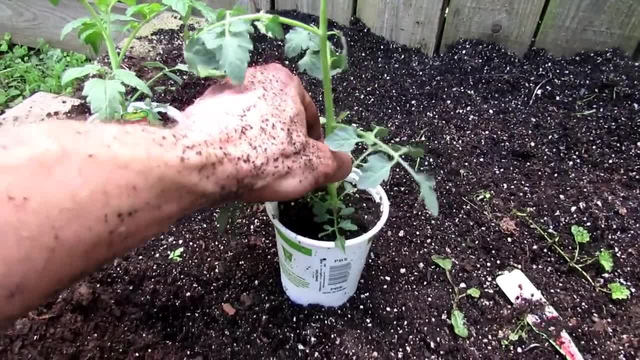 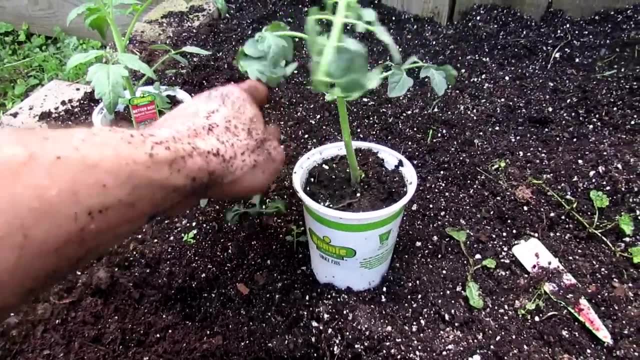 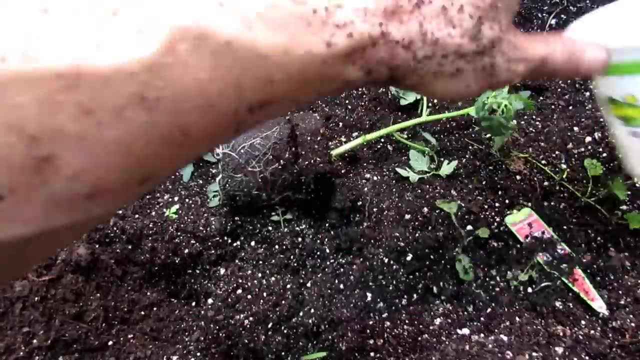 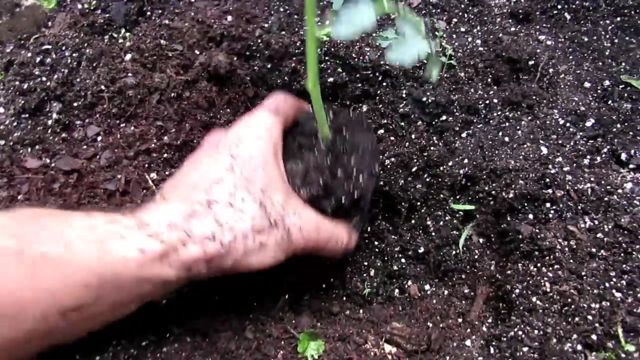 But I thought, since I'm actually doing this as a first bed, I'd show you how to do it: Pinch off the leaves about a quarter inch down- I'm doing this without a tripod- And then gently drop out the tomato And we're going to plant it so that the level of the raised bed gets to about here. 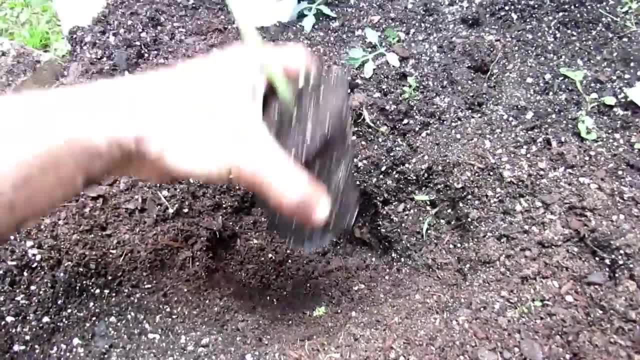 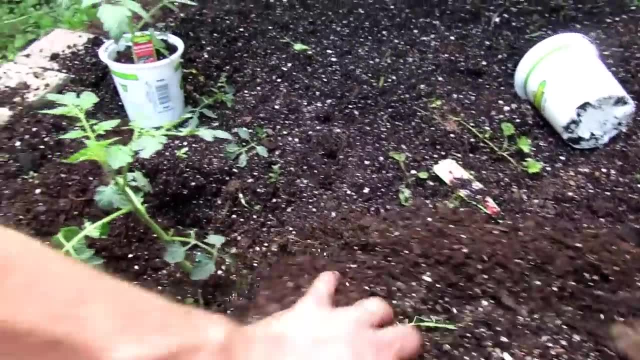 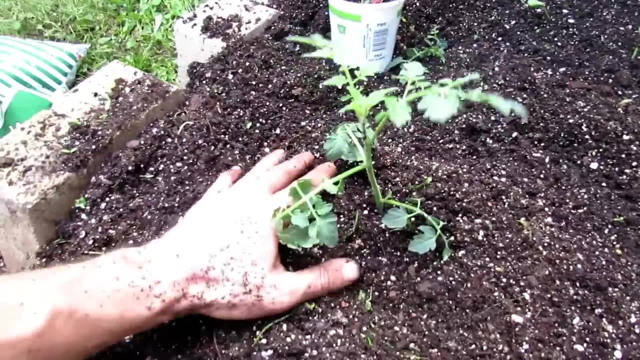 Close to that. Just like that. We set the soil up the same way: Two tablespoons of the organic fertilizer And just gently fill around it. This is the same way that I did the pepper. Once you put it in there, you got your tomato in, press it down around the root ball. 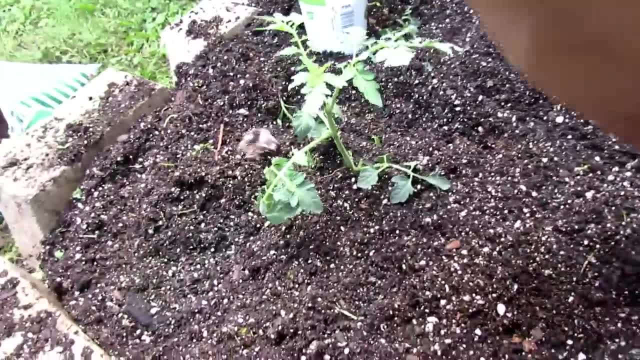 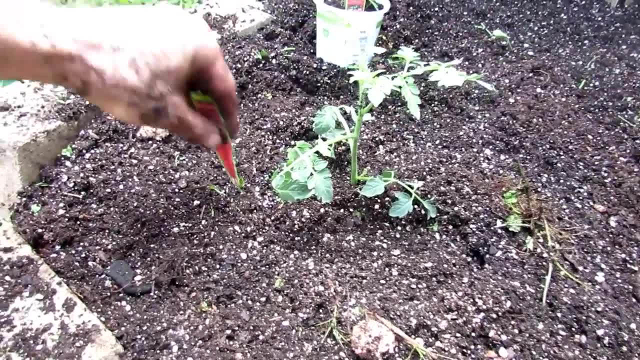 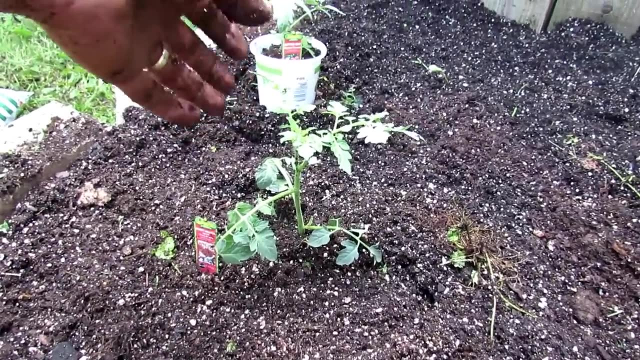 Nice and firm. Bring in some more soil. There we go, That's it, That's it, That's it, And that's all you need to do to get your tomato planted. It's not difficult at all And I really encourage you to go ahead and try having a small space earth bed garden. 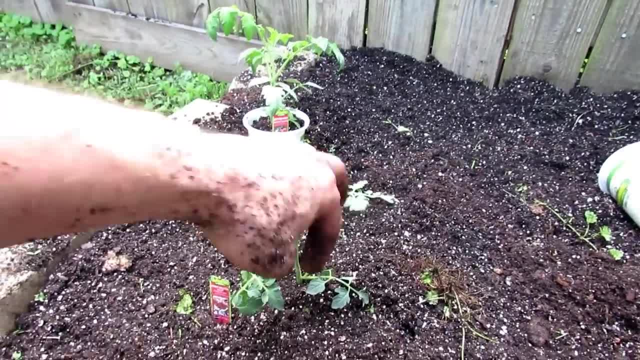 You'll really, really enjoy it And even if things don't go well, you're still going to get a lot of production out of your garden. So I actually I wanted the sweet million over there, but for the sake of the example, 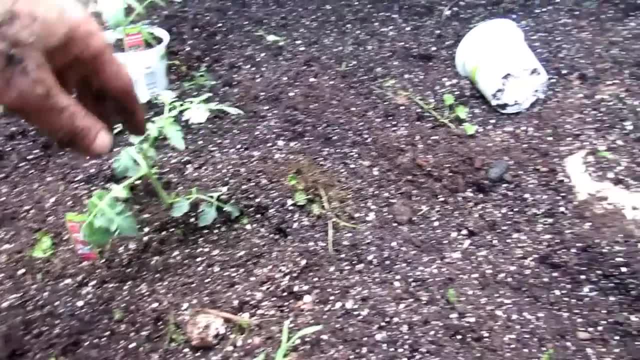 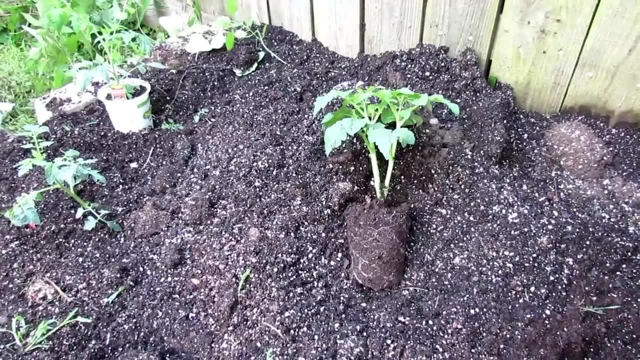 I pulled it over here. So this is going to be a cherry tomato And then I'm going to figure out where to put the other two. But I'll get them into the ground And I'll show you that shortly. Now it's okay to change up your plan a little bit. 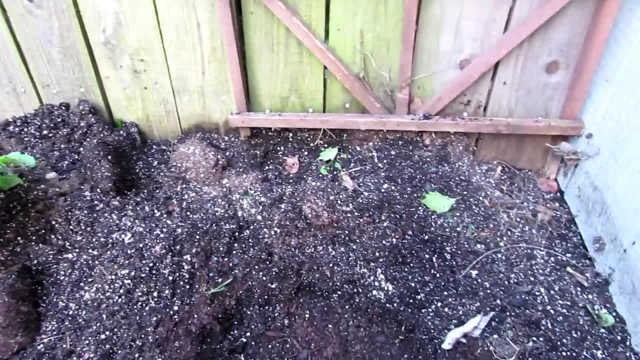 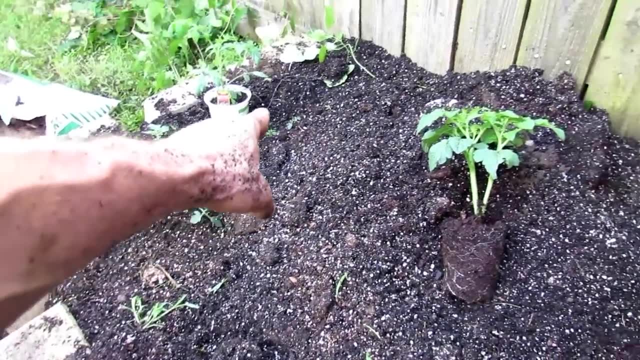 So I'm changing the garden based on the space and the number of plants I'm trying to get in there. Tomato plants will get large, So, for instance, the tomato, I have right, there is going to have space behind it for air to circulate behind it and all around here. 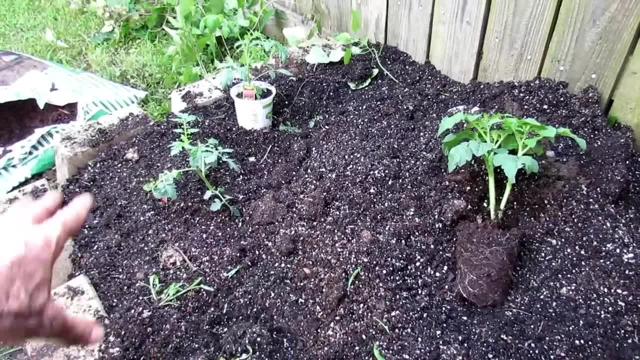 So you want at least a two feet three foot space around it. You can pack them closer if you want, If you have a little more experience and you're going to do some pruning and take care of the plants. But I'm trying to make this. 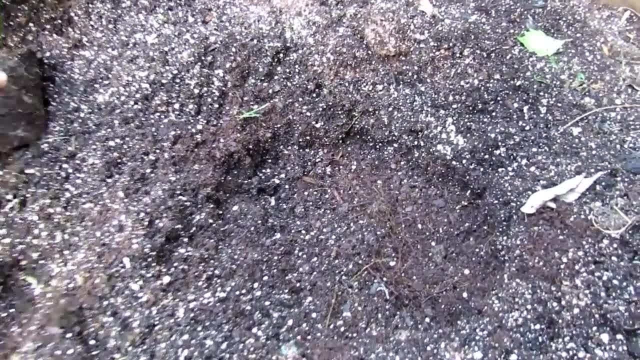 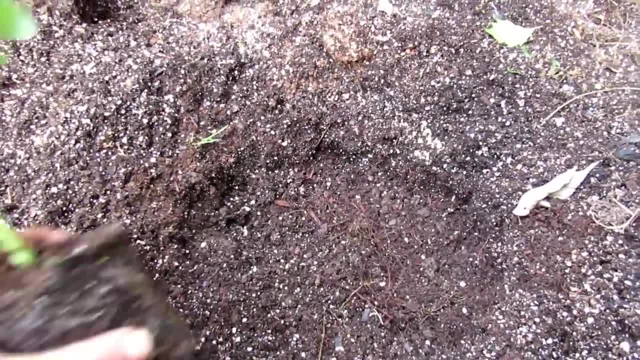 Um, I'm going to show you how I would set it up if you're just getting started Now. this is called a tidy treat. It's a cherry tomato again and it says compact, so it's not going to get quite as big. 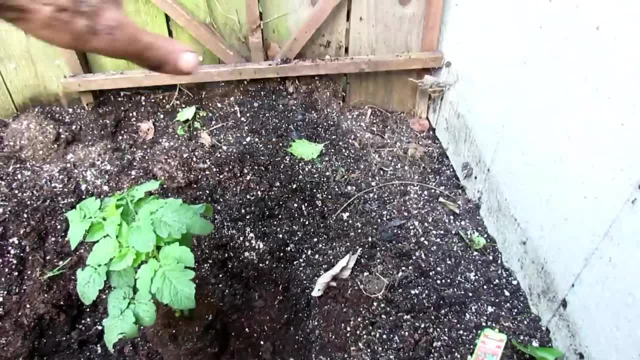 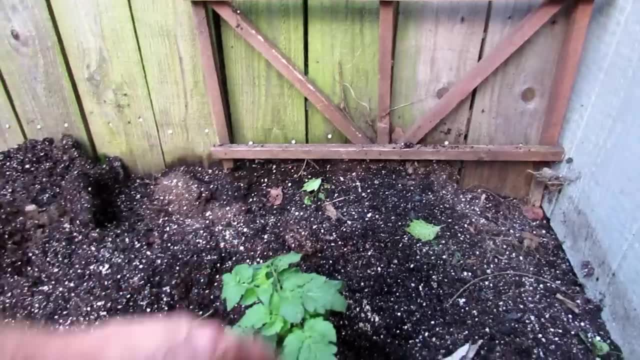 I'm going to put it here with a little bit less space behind it, But this is going to be one tomato plant that's going to take up this whole space. So nothing is going to go over here but the tomato plant. And again you set it up the same way. 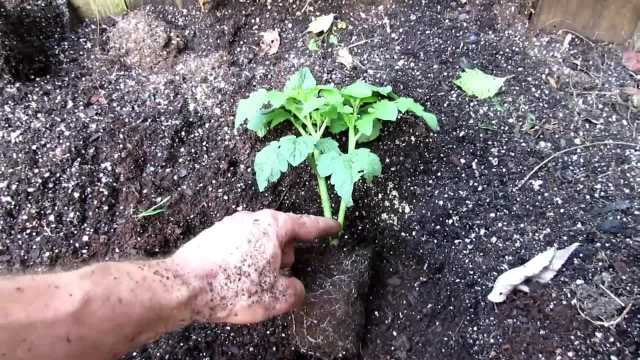 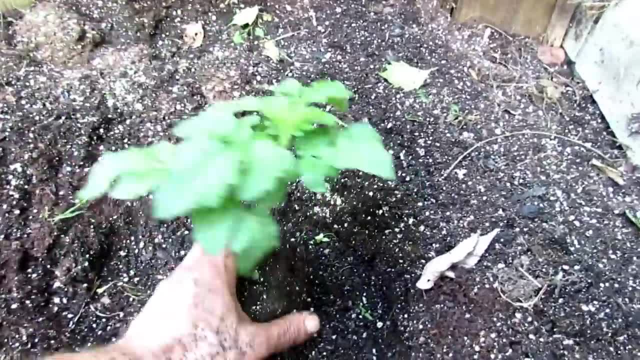 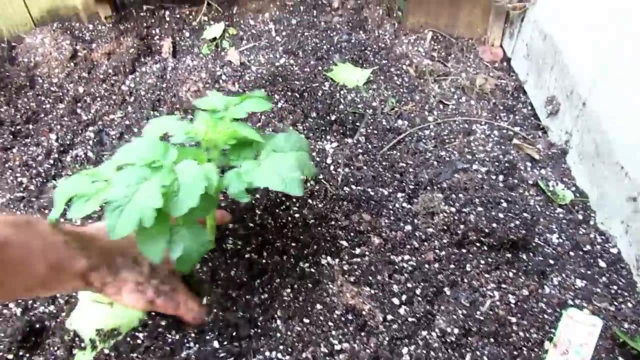 This actually split off into two main stems, but I removed the leaves here and then I'm just going to plant to about there. It'll look like two plants coming up, so I have to raise it a little bit to do that. Just set it in and then move the dirt, the soil right to your plant. 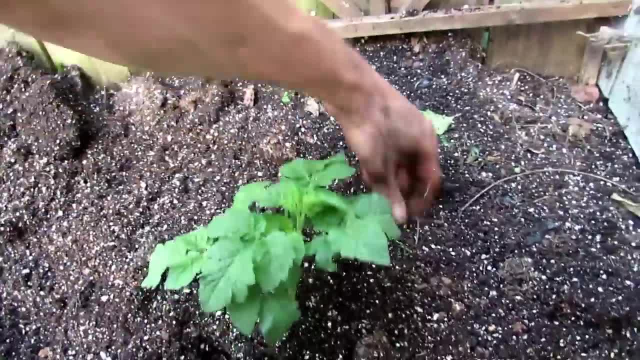 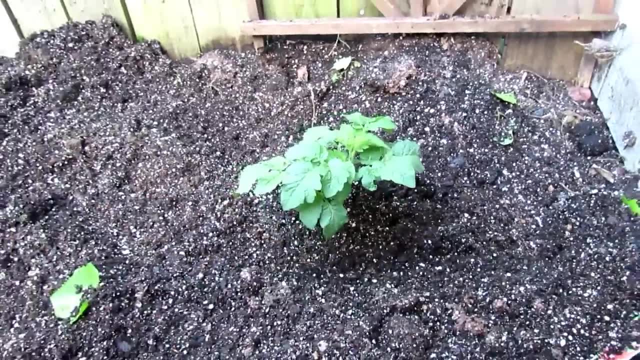 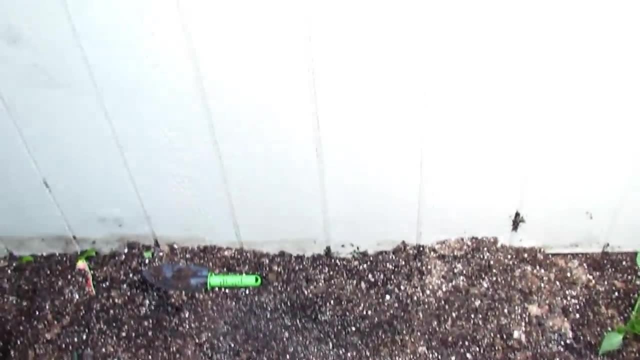 Press it in. You want it to be nice and firm around the plant, so the root system anchors in to the earth, And that's the other one that's set up now. The third one is going to go right here and it'll grow. 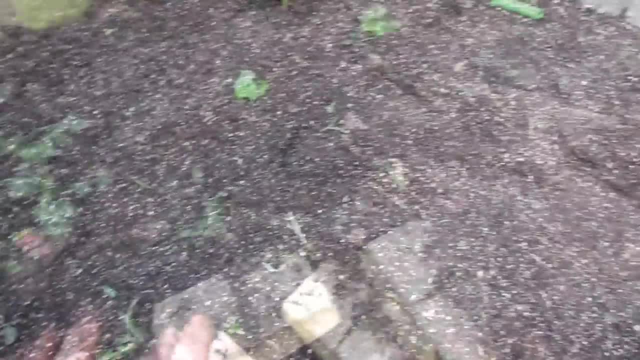 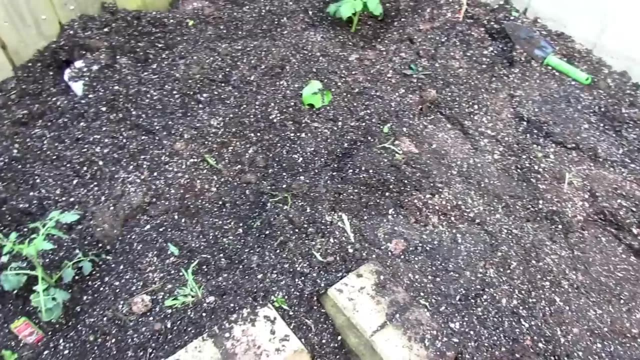 It's got the shed behind it And then the herbs are going to go right in the front seed. They're going to grow quickly. They're warm weather plants. They're going to flower. When they flower, you pull them out and you reseed. 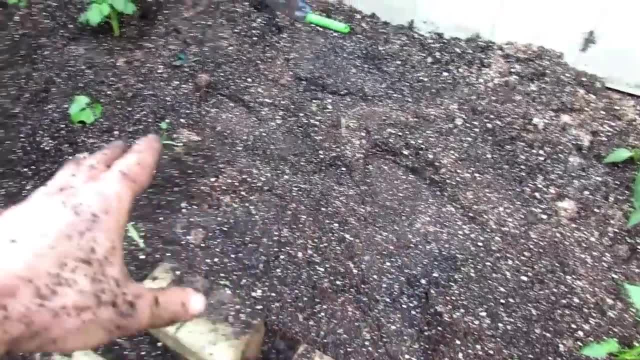 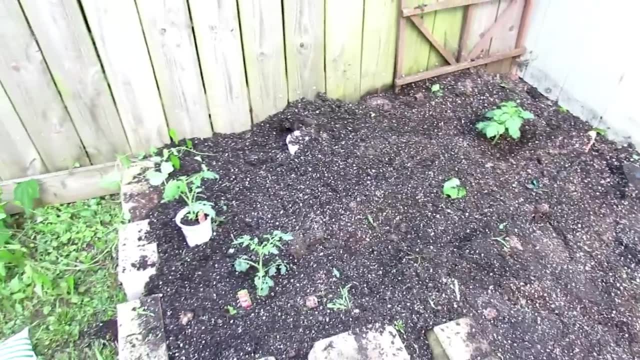 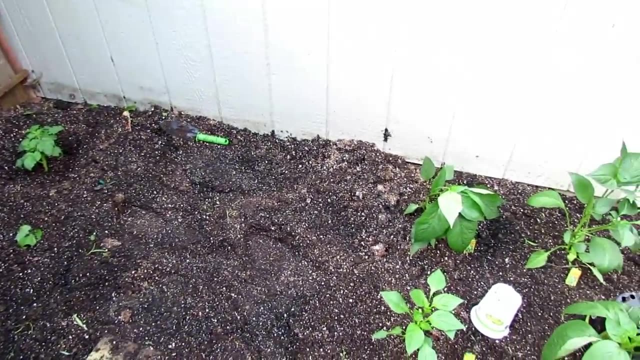 So they're going to all be growing right in here for easy access for cooking with them. And then the oregano is a perennial That's not going to die off. That's going to come back year after year. So I'm going to figure out where I can tuck it in here, where it can just grow year after. 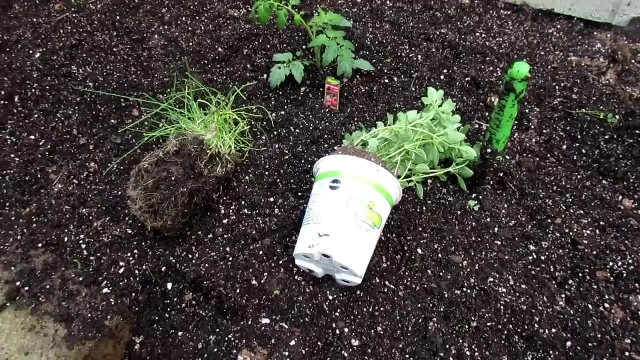 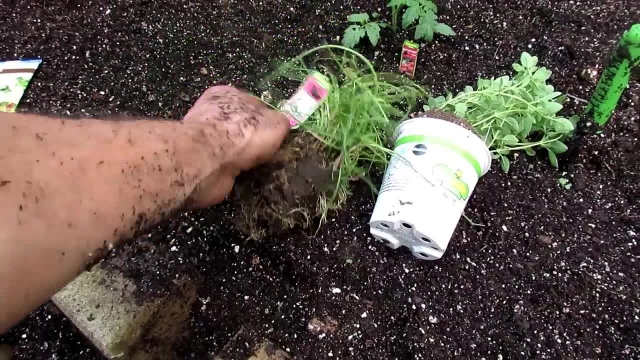 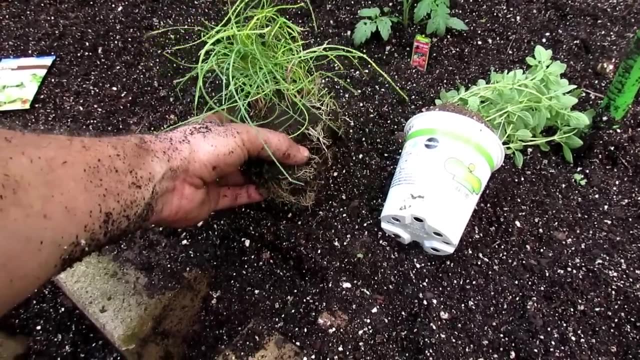 year, So I'm going to put in the oregano. and actually I was walking around the yard, found this from the previous owners: Those are chives. Chives are pretty much indestructible and you can't kill them. So if you are just getting started, plant some chives. 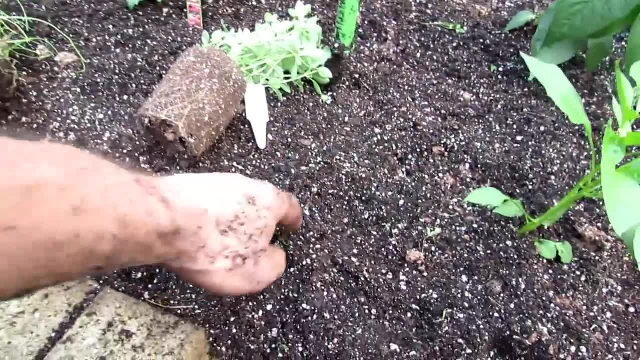 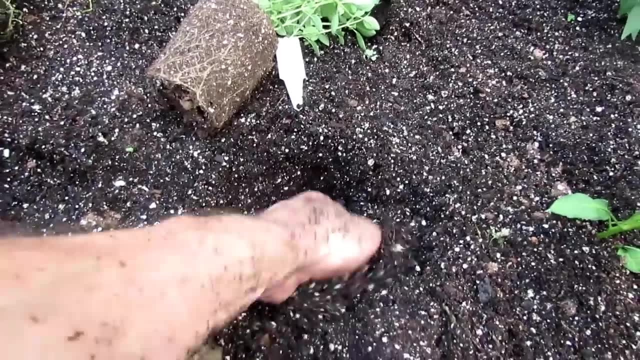 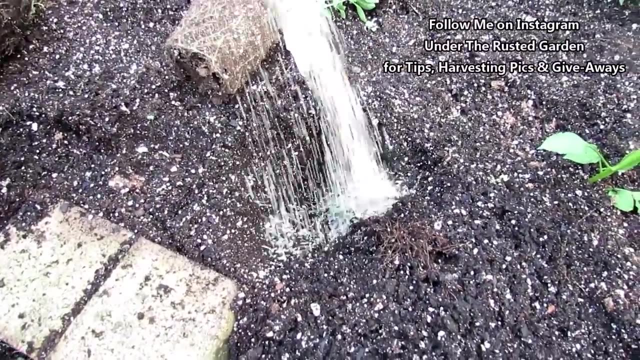 They will come back year after year and they're absolutely delicious with your tomatoes and cucumber salads, And I actually thought for a minute that I was going to be able to put a cucumber plant in here. Sometimes I still get overly ambitious for the space. 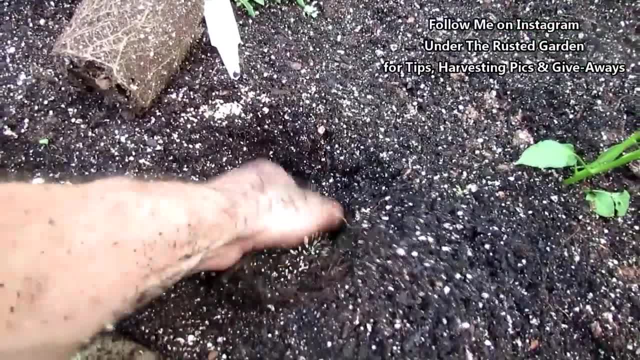 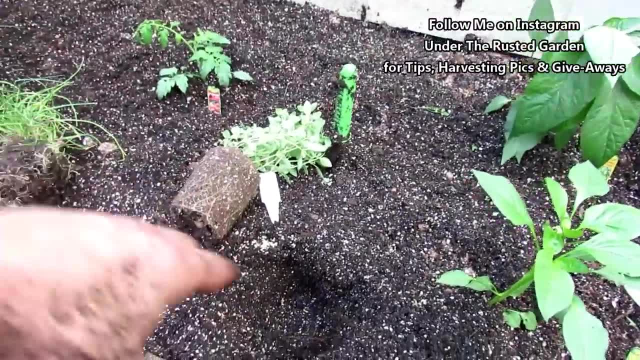 About two tablespoons right into there. The soil is pretty loose. Now, of course, we were kind of blessed there was all this potting mix in here, But you would do basically the same thing I'm doing here for the herbs. They don't need as much setup as the peppers and the tomatoes. 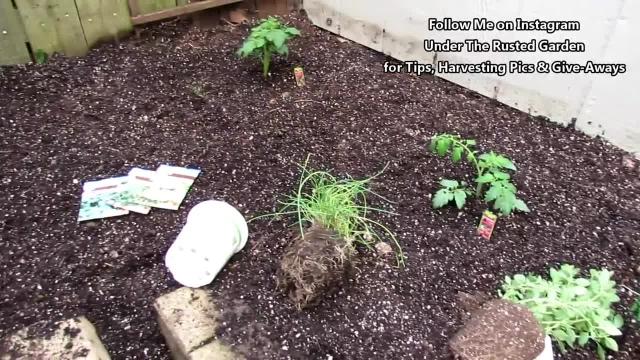 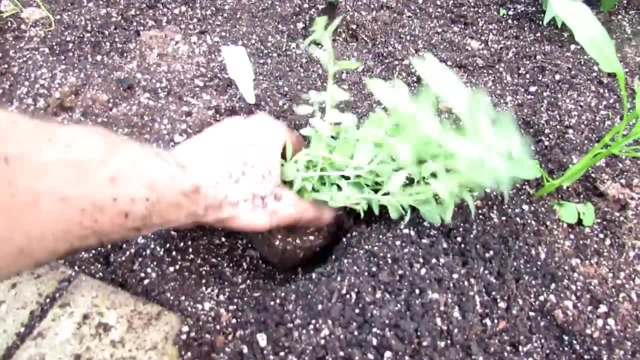 But you would put in your garden soil right into here, Fill up the raised bed, Mix it through And then it's going to be nice and loose And all you do is one to two tablespoons of the fertilizer and then just press the oregano. 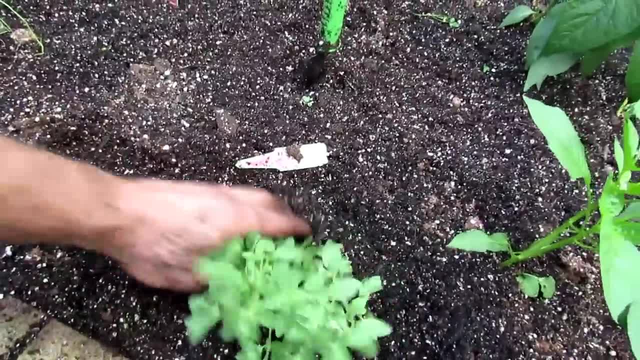 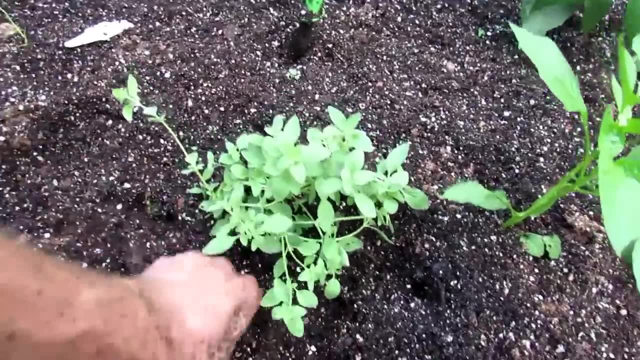 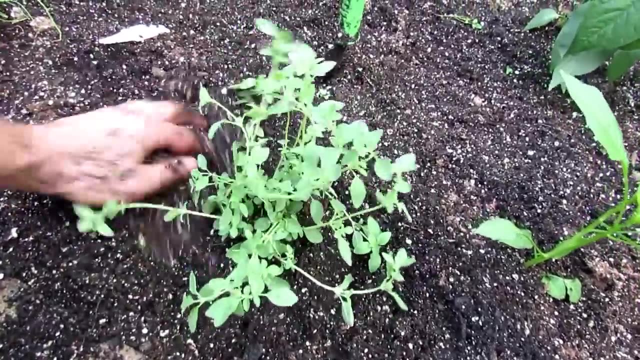 in really nicely. It's alright if the roots get a little bit smashed, But you don't want it to be too fluffy. There is plenty of air space in here for the root system, And this is where the oregano will grow. 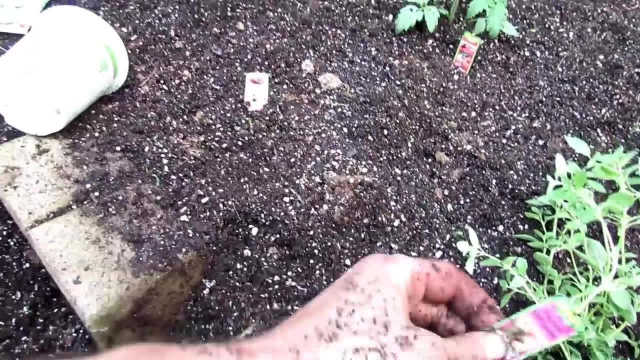 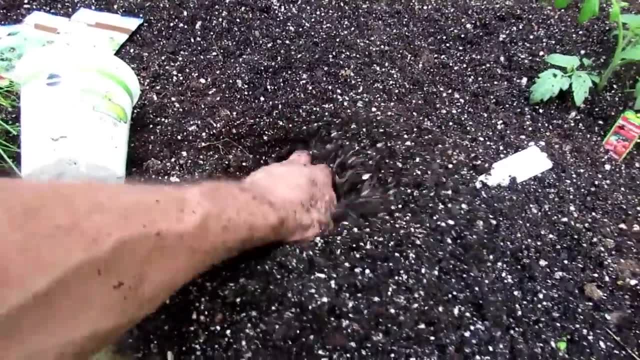 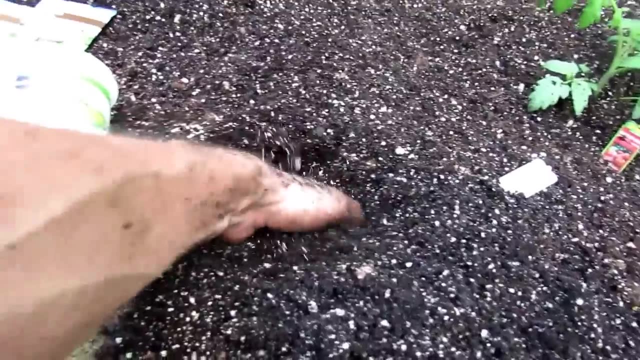 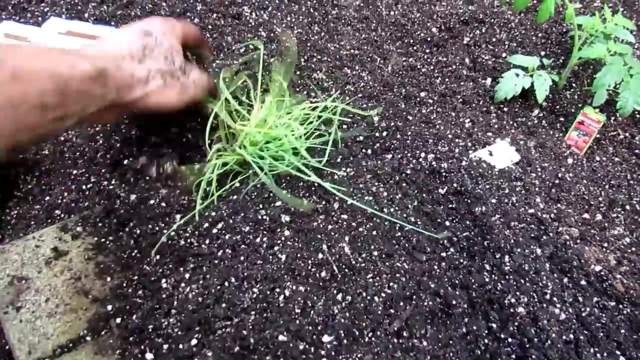 You do the same thing. Space it out a little bit more for the chives. These plants don't take over. You can always trim them back year after year. Dig a hole, One to two tablespoons of the organic fertilizer, Drop it in. 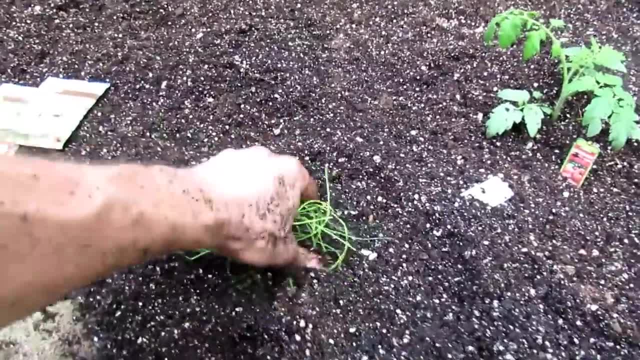 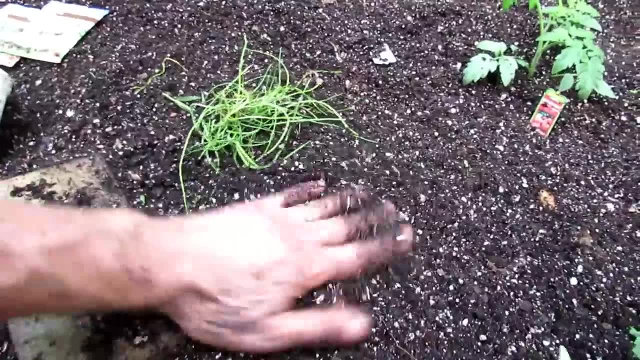 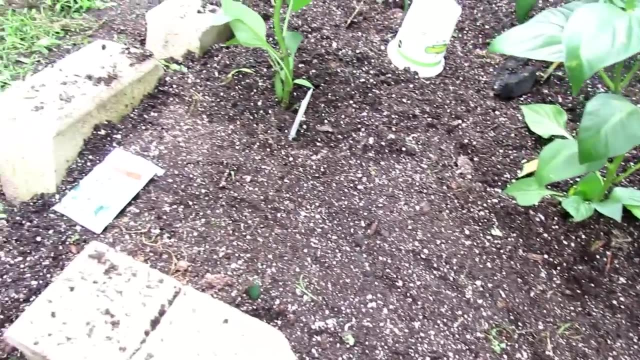 And you can see you don't really need to worry about planting chives. They will take off now that they're in the ground. Alright, let's get to planting the seeds there. Okay, the basil is going to go right in here. 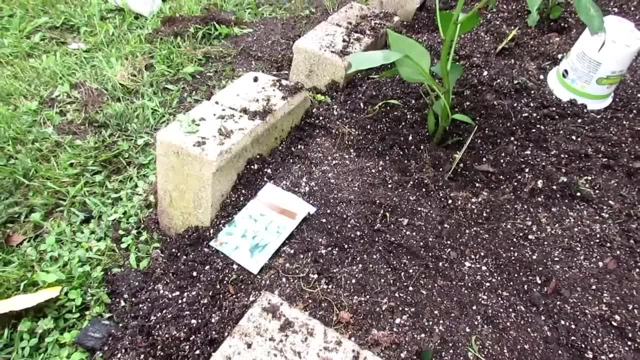 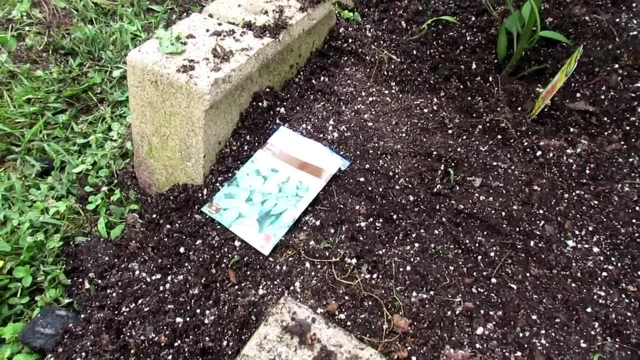 It loves the sun and it's going to be to the front of the garden because behind me is where the sun sits most of the time. Now again, remember, don't go and buy the basil transplants. They're going to be like three bucks a plant. 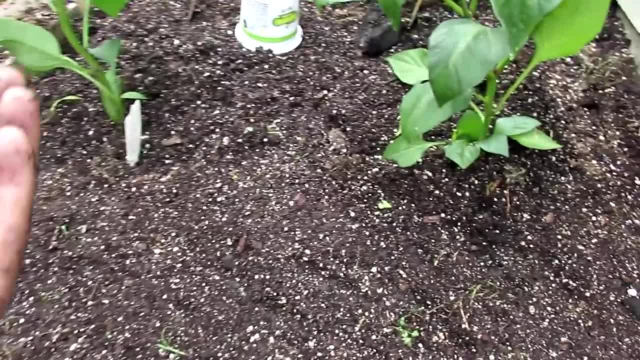 That was like only $1.60 for a bunch of seeds. So to set up the area you don't need to put in any fertilizer, But you want to press the oregano in. Press the oregano in, Press the oregano in. 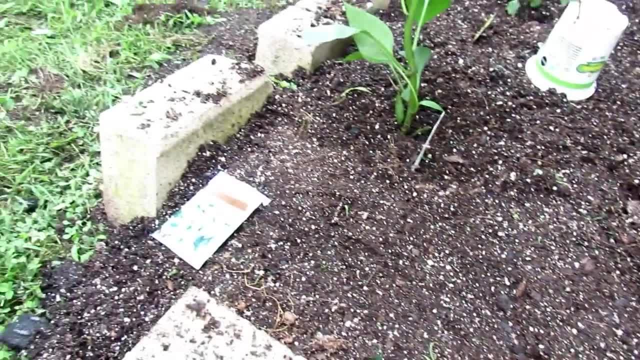 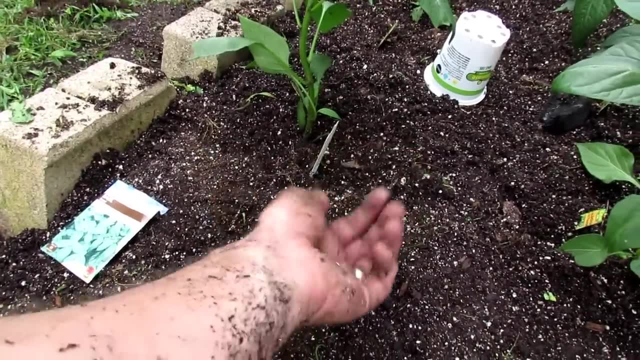 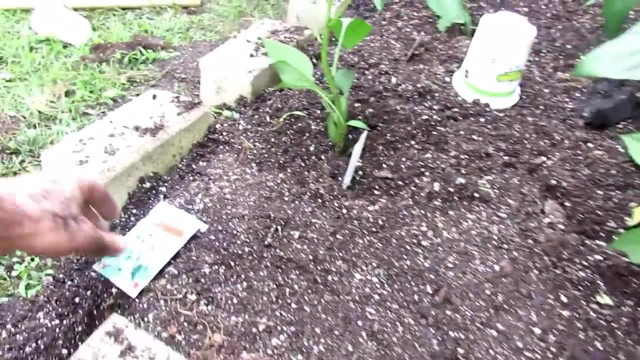 It will make the area down. You want it to be nice and firm all the way across. You don't want the little seeds to drop way down too deep- About 25 seeds, 20-25 seeds- and just sprinkle them into this space. 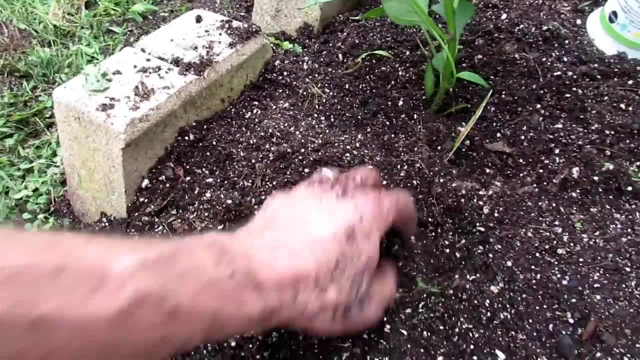 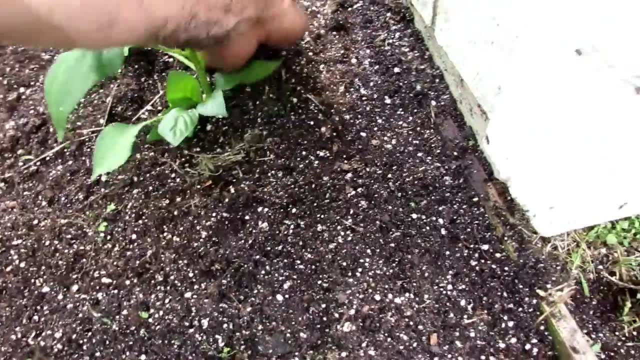 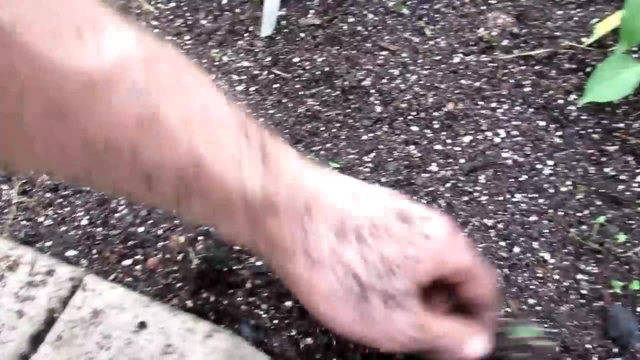 And then you're just going to mix them down: Quarter inch, half an inch deep. This soil is really loose. They're going to grow up through there. just pull in some other soil. every seed doesn't have to come up, you only need about five or six. 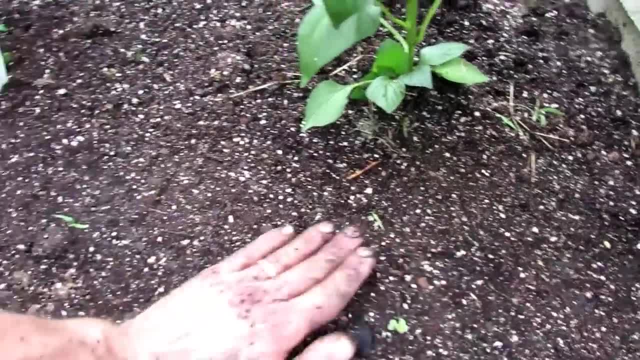 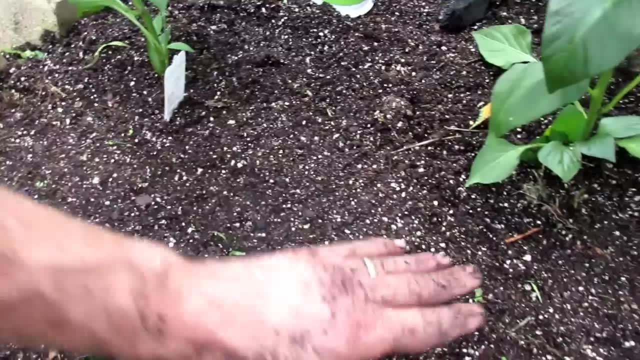 in there, pat it down, and this would get watered in. and again, if you check out my channel, i'll talk more about water soluble fertilizers and how you use those in your garden. but for now these will do perfectly fine, just like that, watered in now, once they come up, once they break the surface. 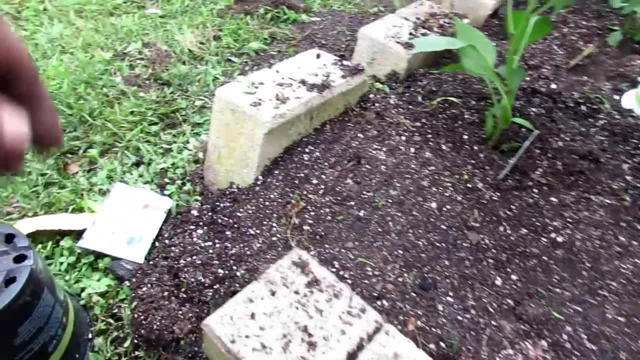 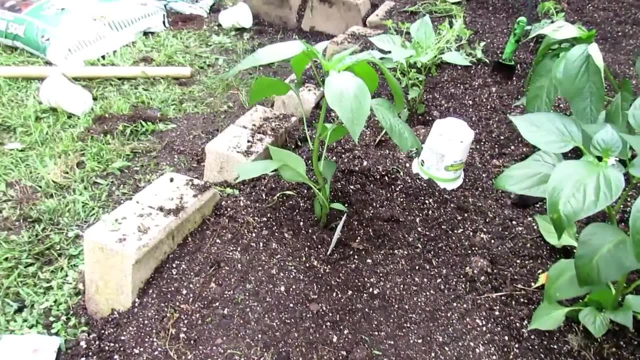 once they germinate, every two to three weeks drop in more basil seeds in a different place, because these are going to grow and then, when they get to height they're going to flower, the flavor changes and that's when you want to pull them out. so two to three weeks after they germinate, 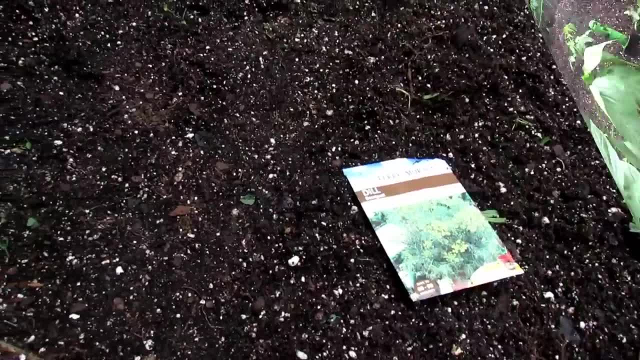 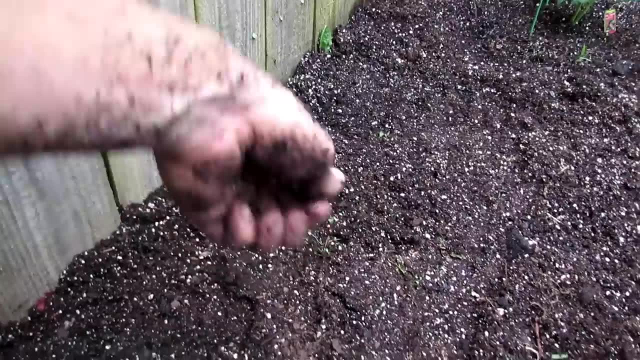 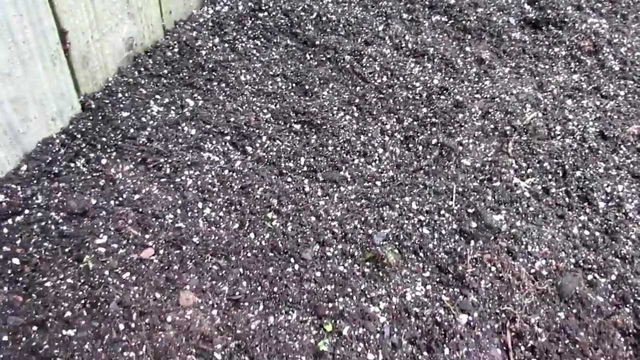 put some seeds in some other places. all right, cilantro, all right. some idea for the dill. it's just going to go in here, pressed it down, about 20 or 30 seeds and just sprinkle them in all over, mix everything up nicely, about a half an inch deep, quarter inch deep, it doesn't really matter. 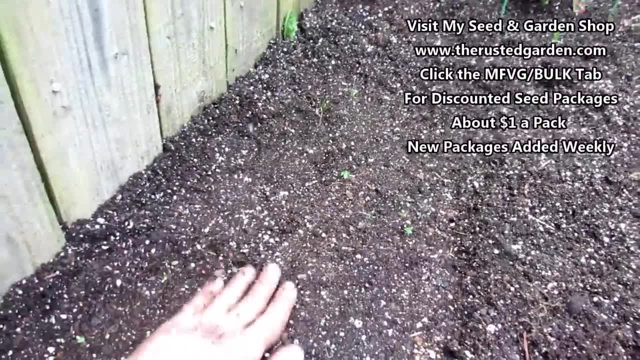 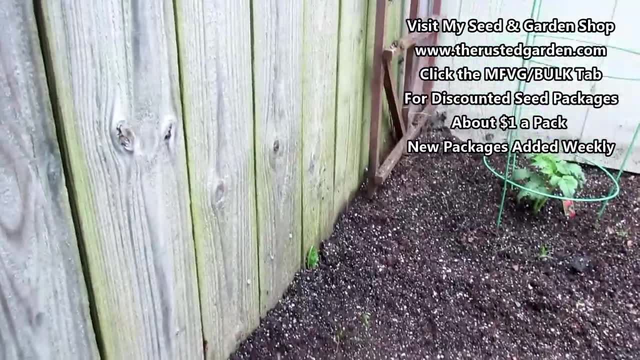 and then press them in. dill grows quickly now when these all come up. if there's a lot of them- about every six inches- you want to plant, so just thin them out. but the dill is going to grow here and it gets quite tall. i like to let it flower and actually collect the seeds again, and if you 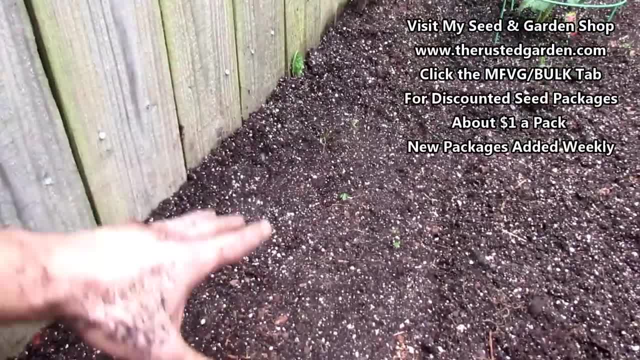 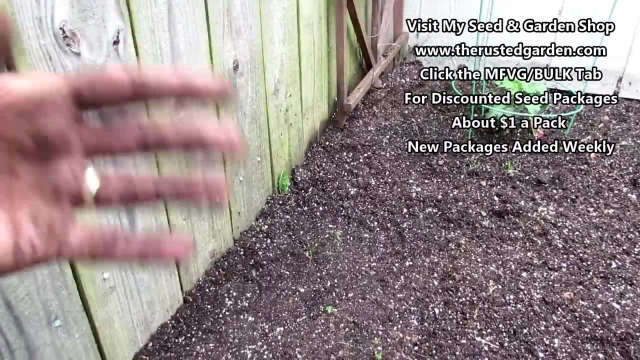 just let it do that. it will drop seeds and it will come back year after year. but this will be growing behind the tomatoes. you know, as the season progresses the tomatoes will fill in this area. the dill might get blocked out a little bit, but that's what you do in small spaces but you'll get plenty of dill production. 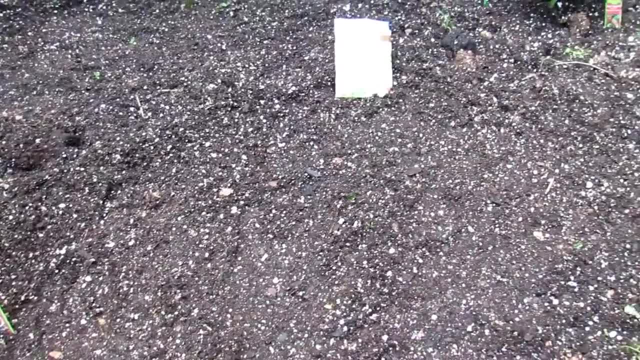 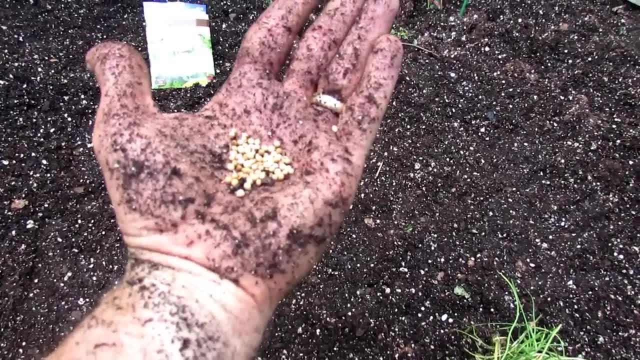 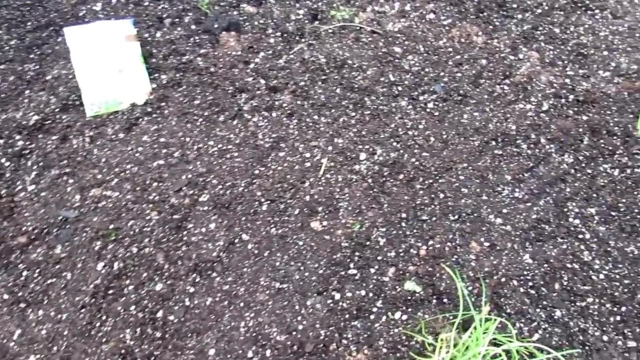 out of here to use in your garden. and then, finally, the cilantro will go in- a lot of cilantro- right into the space, and cilantro are actually pods, so in each one of these are a couple of cilantro seeds, but we're going to fill in this whole space. sprinkle it through just like that, if you like. 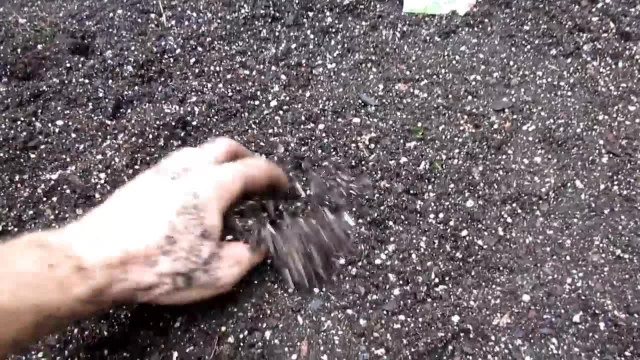 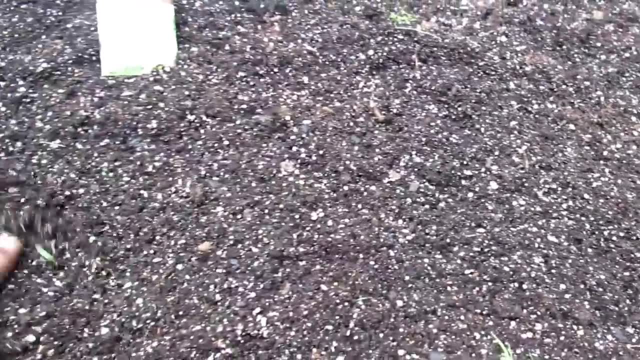 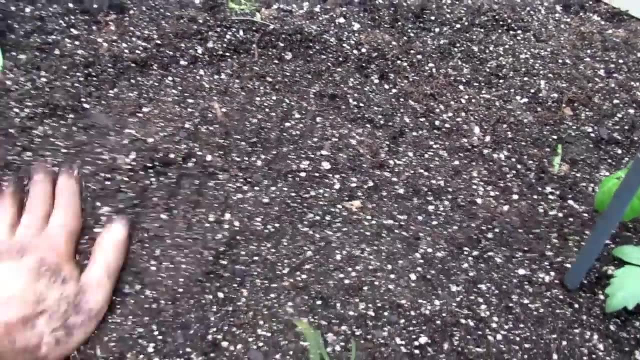 cilantro. you're going to want a lot of cilantro, so don't just grow one plant, because when you go to pick it you're going to probably take the whole plant. so put a lot into this space. half an inch down, quarter inch down again, the whole area was pressed in and just pat it in, water it in and you'll have. 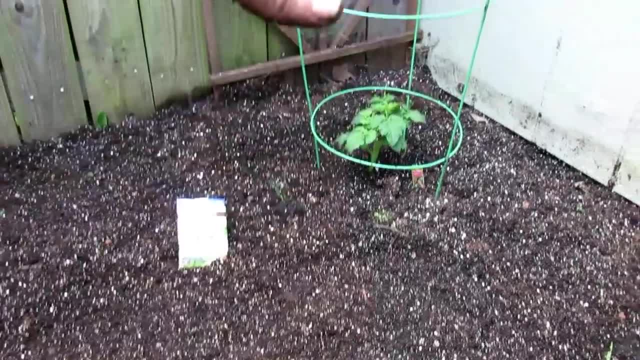 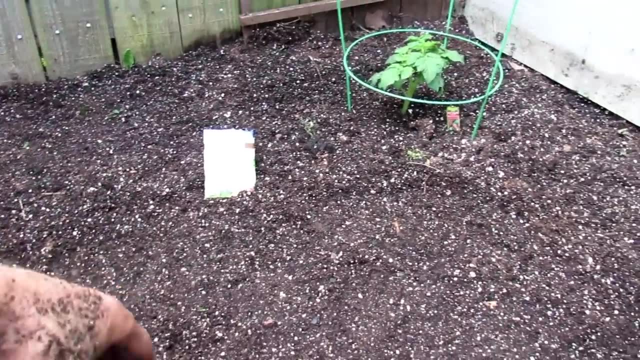 plenty of cilantro, and cilantro again will get tall. it's in front of the plants. it's going to get about this tall. when it starts flowering, the flavor changes. so again, two to three weeks after this is germinated, you might want to drop seed in another place and then, when this begins to flower, 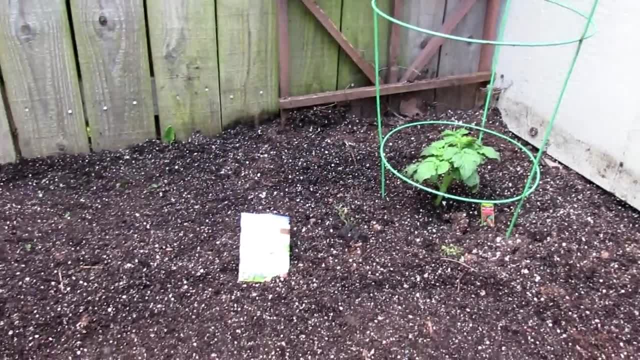 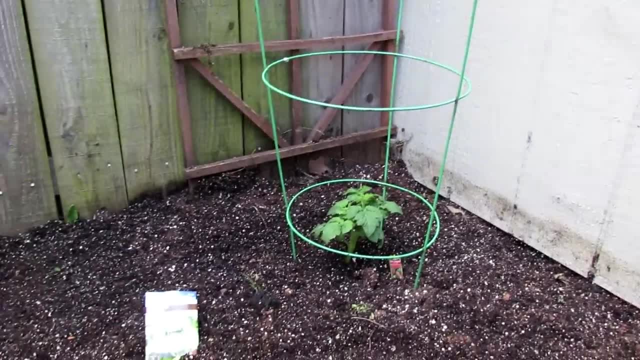 pull it out now, like if you like coriander, that's what cilantro is. you save the seeds. i hope i got the name right. i always forget stuff. but you can save the cilantro seeds and use them too in soups and as an herb. 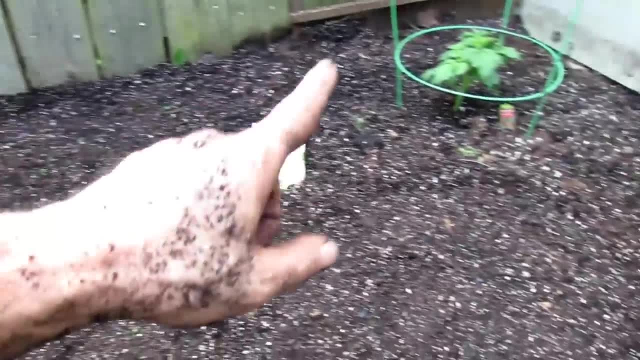 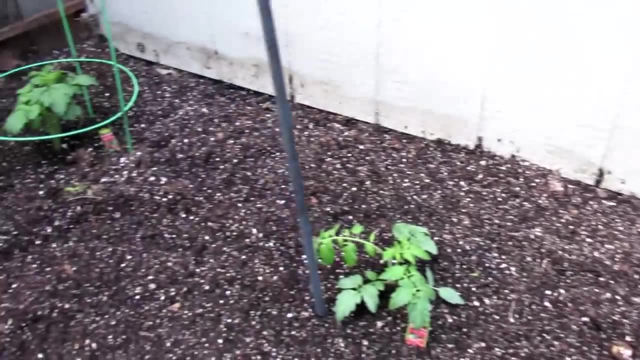 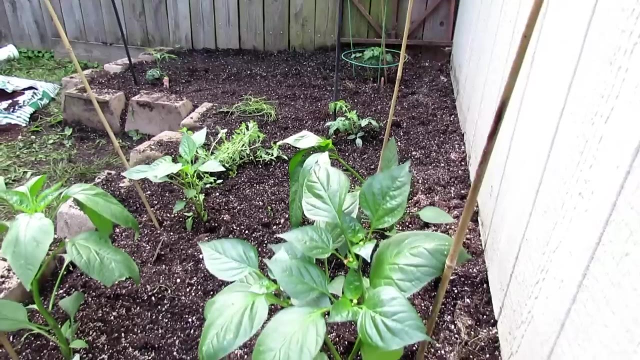 differently than the leaves. all right, we have dill in the back, cilantro right here, basil over there, and now we will get to the top dressing and the staking of the tomatoes and peppers. the steaks are in. i'll talk about those in a second. you want peppers and tomatoes to have something. 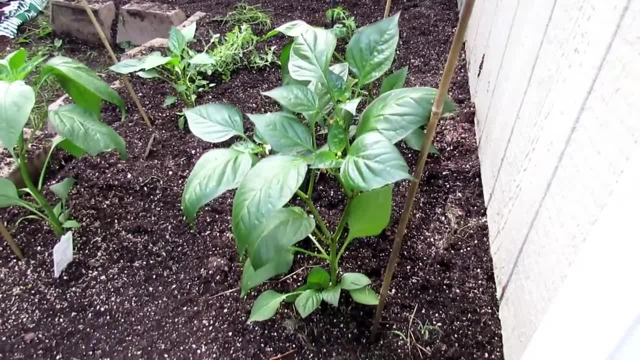 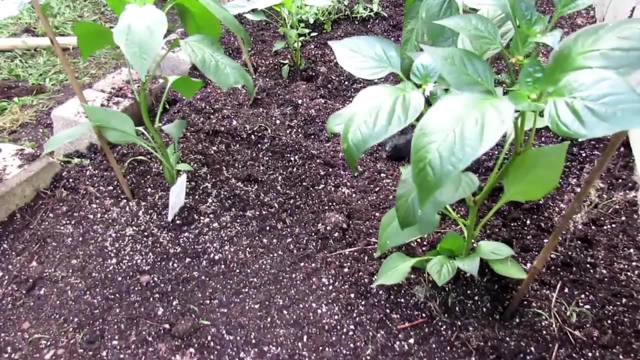 to climb on, because the peppers are a bit fragile: when they get heavy with fruit they're going to break and the tomatoes or vines are going to want to sprawl all over the ground. so you stake them to control their growth. so about one tablespoon of the organic fertilizer? just sprinkle it around. 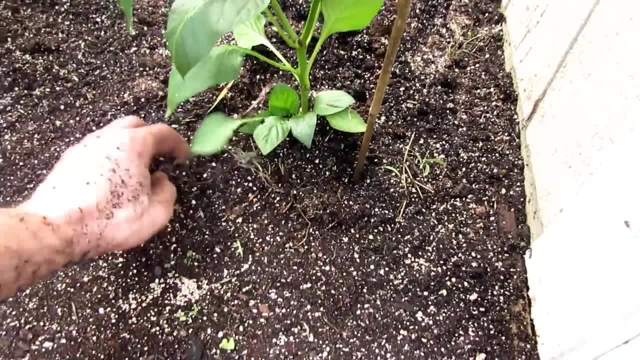 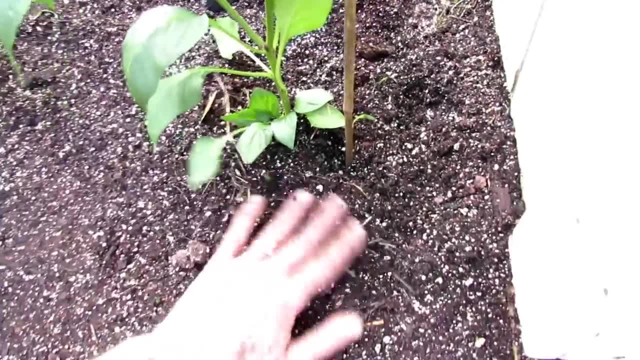 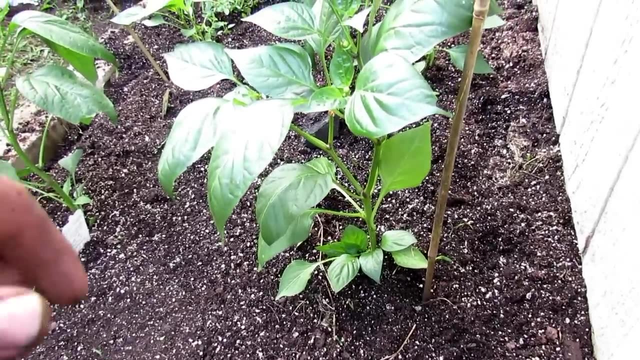 the plant. you want to be about one, two inches away from the stem. scratch it into the surface. the basil i just planted there is going to get a little food and scratch it in. so we've got the granular type fertilizers, which are insoluble. check out my videos for more about that. but that 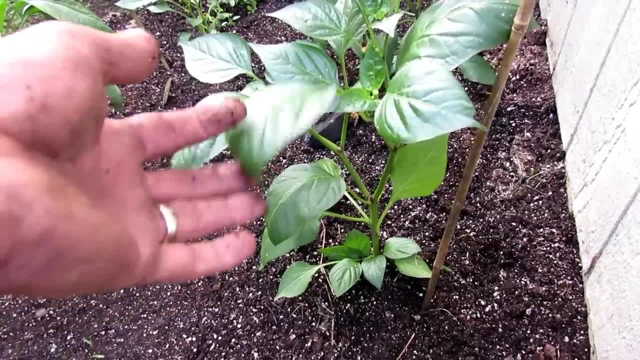 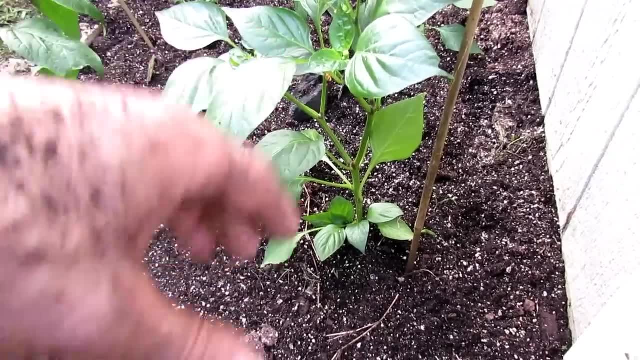 means that the soil life has to break that down before the npk is available to the plant. but that's what you want to do. the plant's going to grow with what mpk is already in the soil- nitrogen, phosphorus, potassium- and then the organic fertilizer will break down over the weeks and it'll be available. 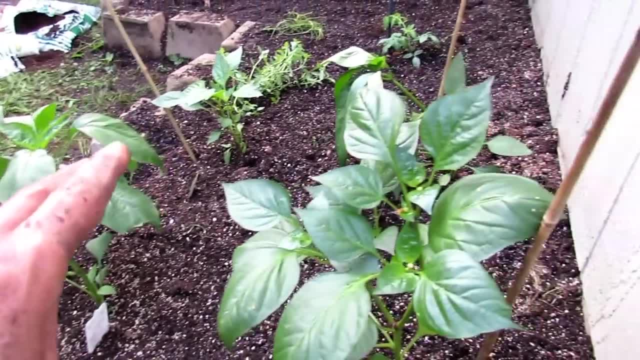 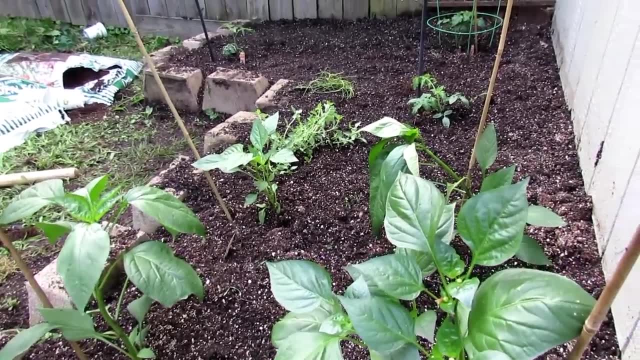 for the plants to grow. so all the peppers will get one tablespoon sprinkled around, like that same with the tomatoes. probably do it around the planted chives and oregano. you don't do that for seeds that you drop. you really just want to leave the. 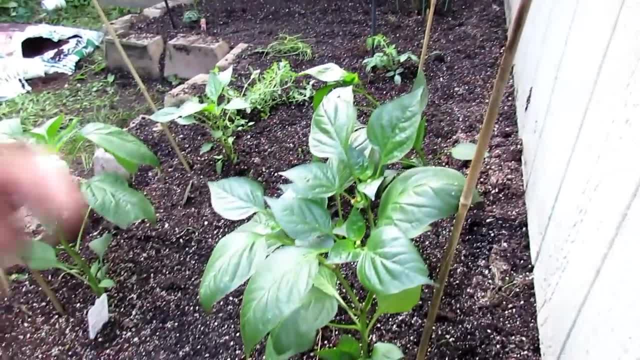 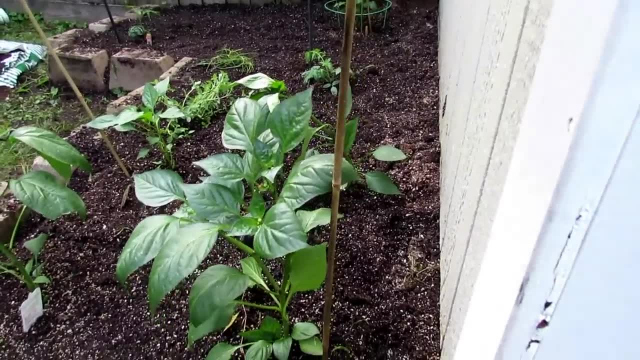 seeds there and let them grow water soluble fertilizer. you can check out my channel again, like i said, and see how you use that. so the stakes: bamboo poles. these are about five feet. this is all you really need for a pepper plant, and notice that i angled it towards the shed. the 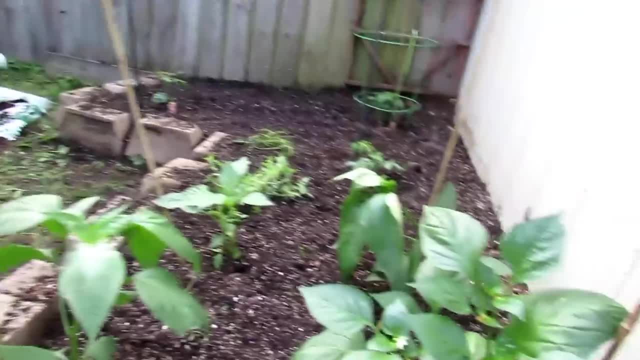 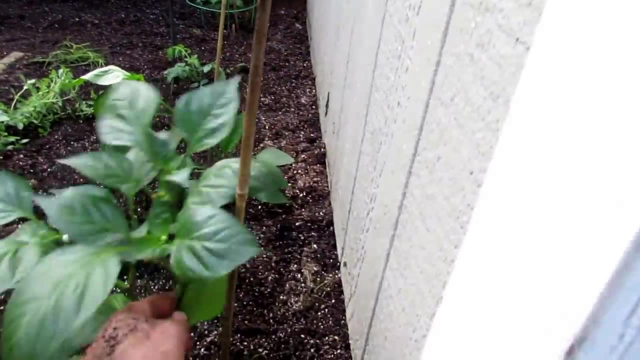 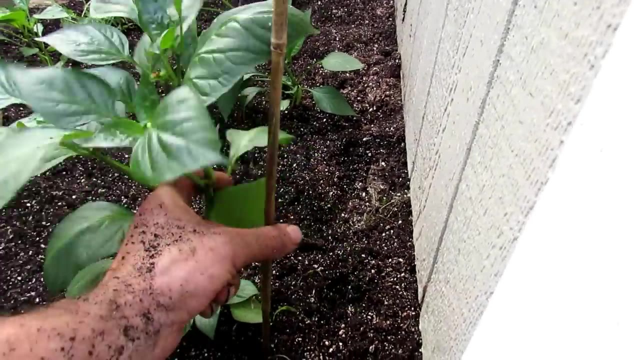 ones over here. i angled out to the left. that's just so that the plants will go out to open space. that's only back up to one, and i think the plant will hold up very well because it will grow everywhere. if it does, that'll be good. if it's not, uh, it's not as good. it's just not easy, because 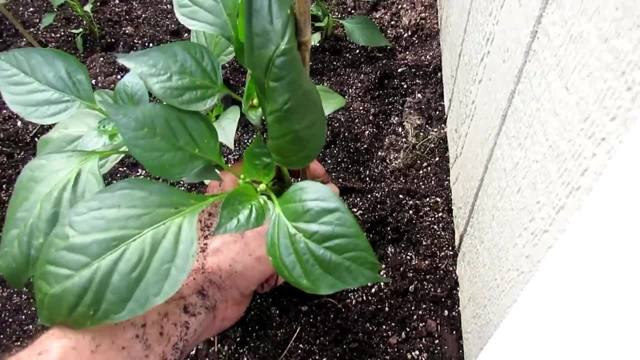 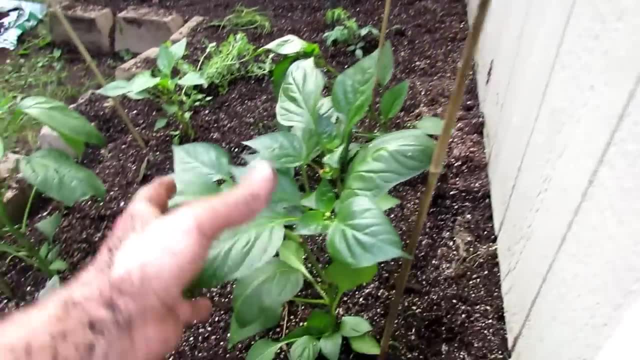 like i do. i like to keep my plants in the air so we don't let the air in when we start growing, and i like to use a twine like this. you can have a little bit of a hole in your plant so it can help support your plant, so you can have more sunlight and air can circulate right through. 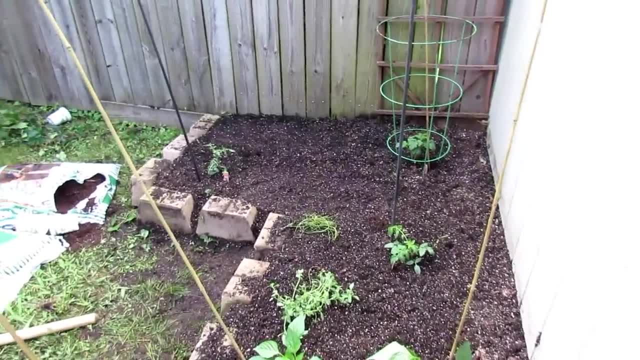 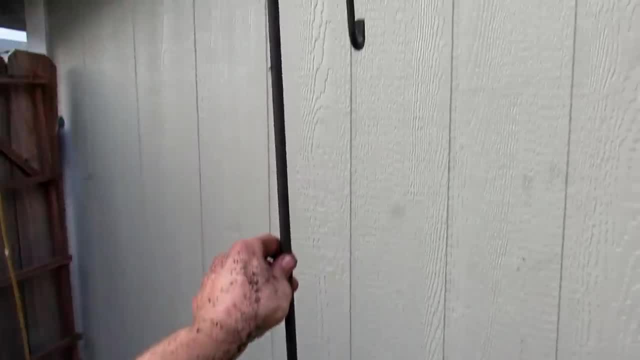 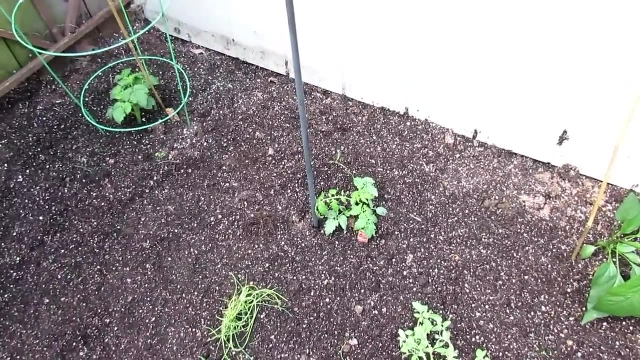 there as the plant grows, you're going to just take some string and tie it big loop around it, don't garden. I was able to find these. these are for hanging plants- and I just dropped that in and secured it. you know, down maybe about a foot and the tomato plant. 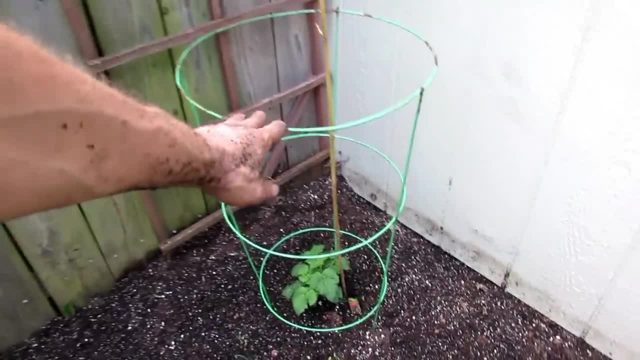 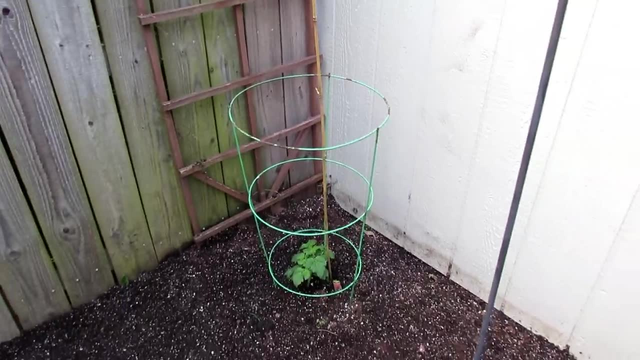 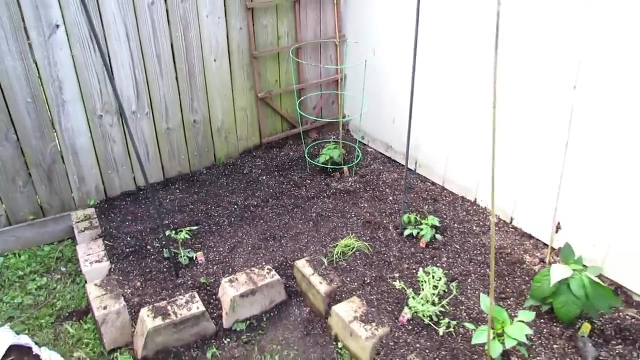 will grow right up that. they also had a tomato cage. this three circle thing is used for caging your tomatoes, but this will get bigger than that, so I did drop in a bamboo post enough. anytime your plant starts getting bigger, you need another post. go ahead and drop something in, but this is the space planted with. 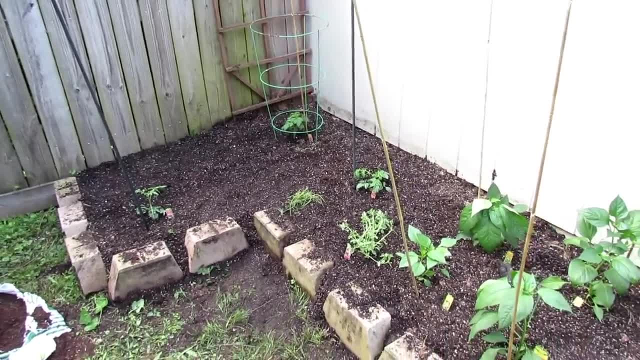 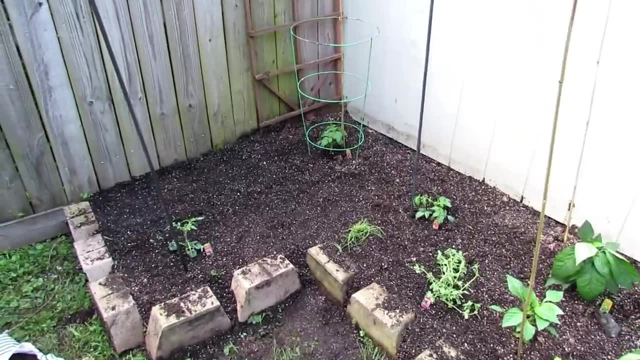 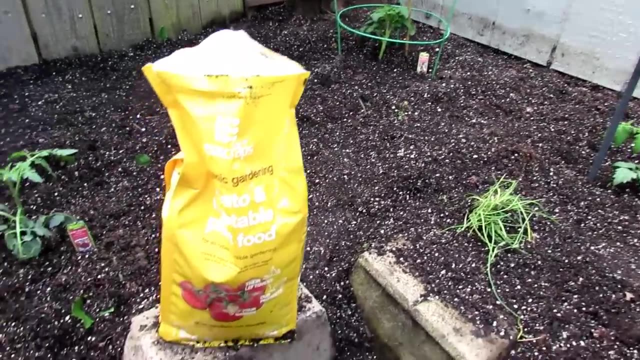 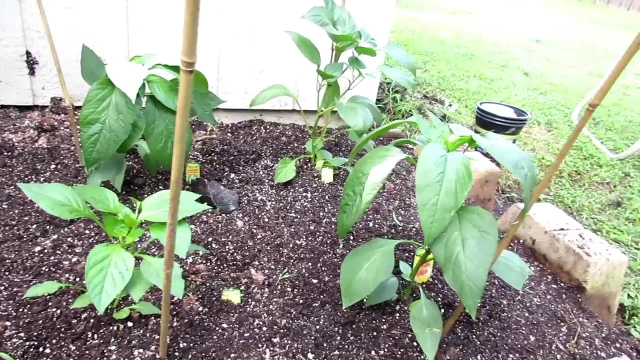 four peppers, oregano, chives, three tomato plants, basil, cilantro and dill. all right, so after it's been top dressed, everything's staked, everything's planted, you're gonna water it in, but I just wanted to show you by doing it this way. it's not that expensive. it takes a little bit of work, but we concentrated. 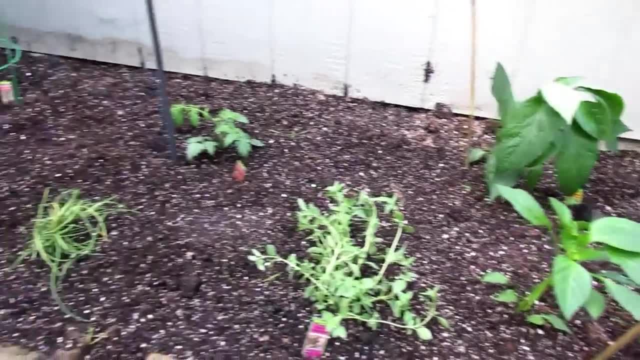 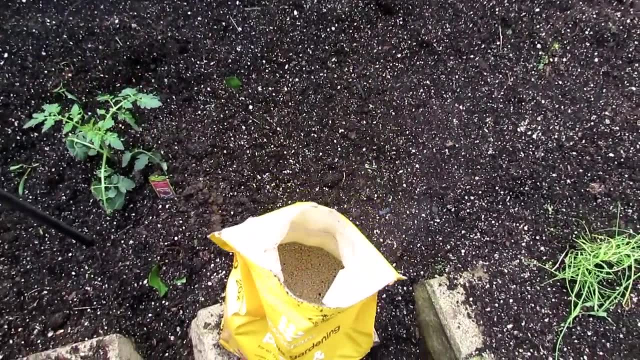 all the resources right to the planting hole. plenty of fertilizer left. I think that's about it, and I'm going to show you how to do that in just a few minutes. I think this was six or seven dollars a bag, four pounds, and there's plenty of.